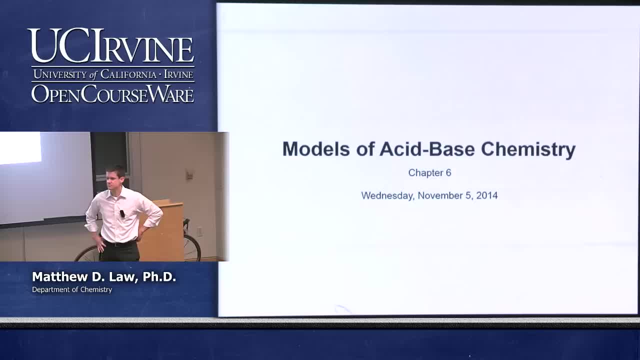 on the exam. So the exam is only Chapters 4,, 5, and 7.. So our discussions of acid-based chemistry today and on Friday will be on the final right. So that's where it will be picked up for testing purposes, So you can relax about not having to cram. 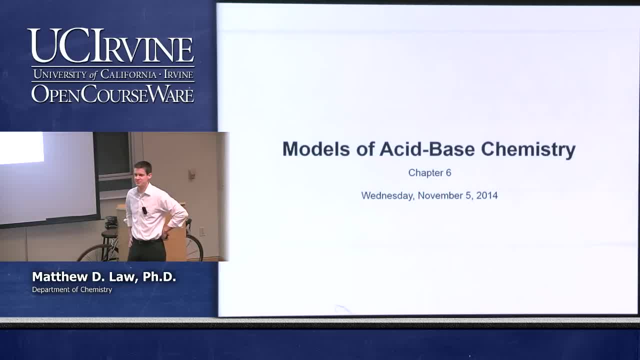 an additional chapter down your throats, you know, in the last few days before the exam, which is completely unfair, of course. So relax, try to enjoy this a little bit. here We are revisiting, in some senses expanding on the subject, which is basically an old friend. 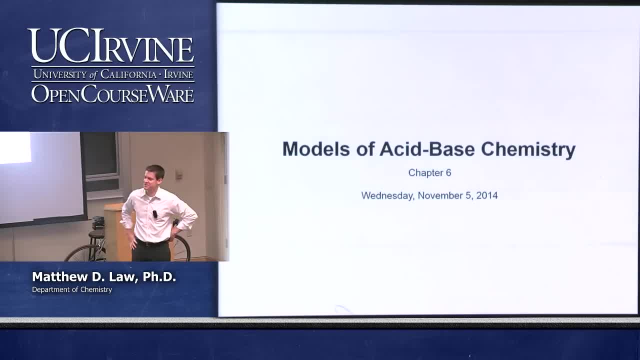 to all chemists right: Acid-based. there's always an acid-based chapter in every chemistry textbook, right At least one. So what we're going to do is we're going to kind of expand on some of the concepts that you've learned about in the past and apply it, of course, to the inorganic. 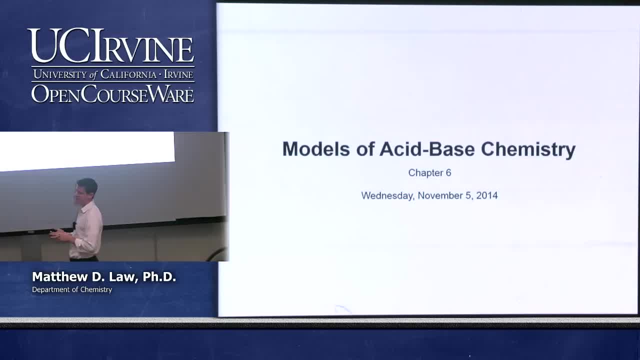 problems that we're interested in. So, in particular, using things like MO theory and acid-based chemistry, combining those kinds of concepts and trying to come to some sort of more thorough understanding about how acid-based properties are measured for inorganic species. So today, 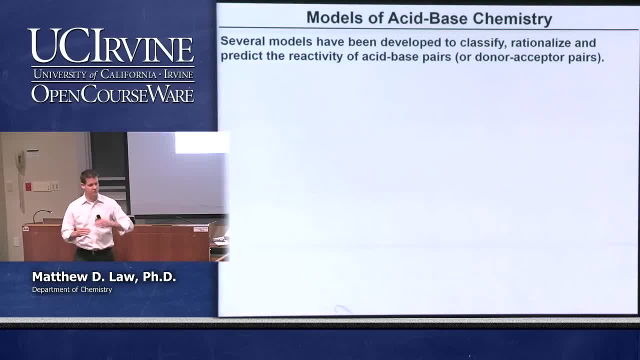 we're going to look at some examples of acid-based chemistry There are. if you look through the history of chemistry as a discipline, there are many, many different takes on what an acid and base is right. This is a very common, ubiquitous kind of reaction And so 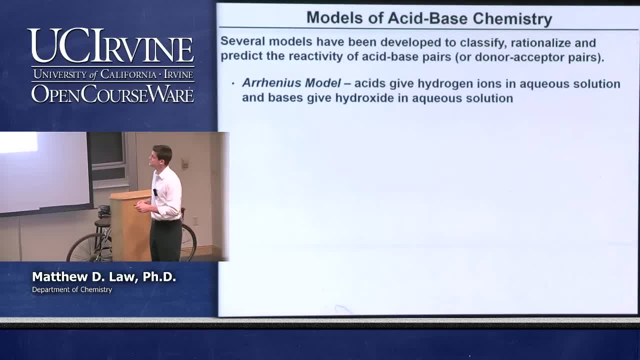 we can look through kind of the annals of history here and see a number of different models, some of which we're very familiar with. So Arrhenius model is always discussed in gen chem right, And so the Arrhenius model around the turn of the 20th century it was. 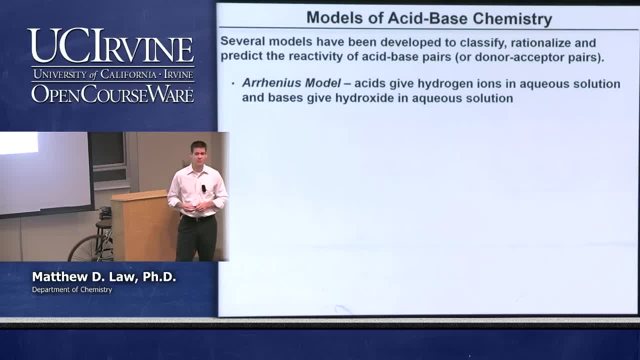 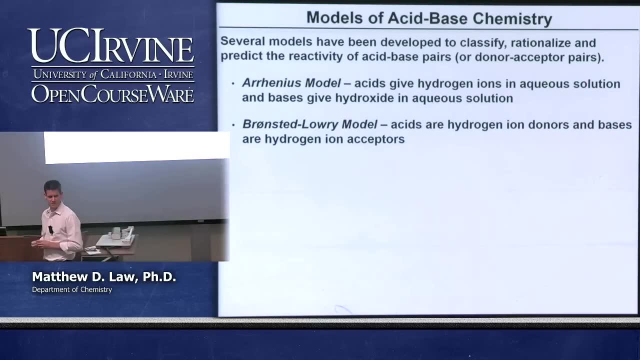 basically acids give hydrogen ions in aqueous solution and bases give OH- in aqueous solution. So it's a very much narrow definition focused on aqueous chemistry and looking at proton and hydroxide Next. the next really big model that stuck was in the 20s. This is the Bronsted-Lowry. 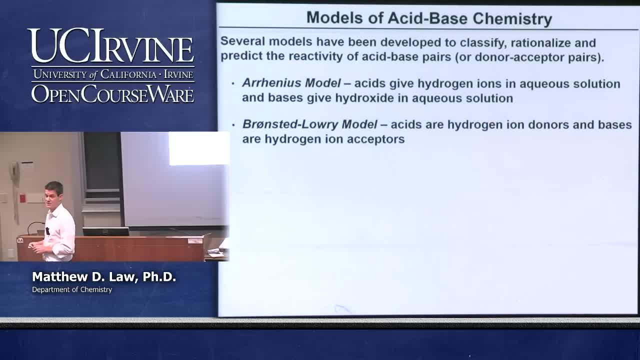 model- and this is, of course, the most talked about model in gen chem, where acids are proton donors or hydrogen ion donors, and bases are proton acceptors- hydrogen ion donors. So we'll briefly revisit this, bringing us to the Lewis model, which was actually around. 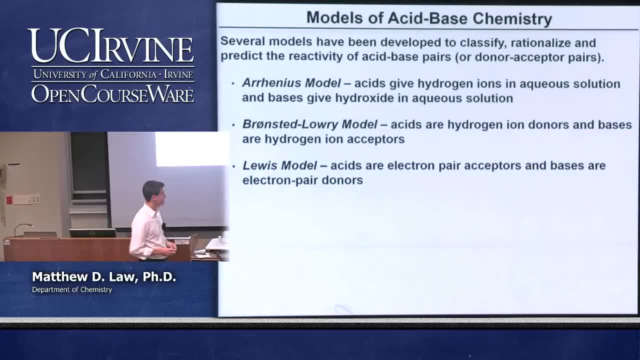 the same time as the Bronsted-Lowry picture came out, And the Lewis picture is the one that we're going to focus on the most because it's the most general of the three that we've put up so far And it also has a lot of applicability to inorganic species- Acids in the Lewis picture. 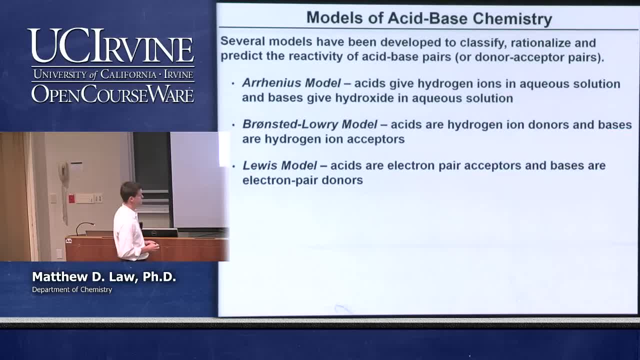 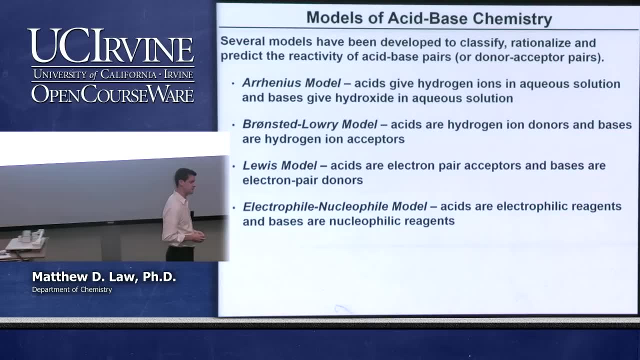 are electron pair acceptors and bases are electron pair donors. So these are familiar models. There are many others, some that are around with basically the same sort of concepts, just a little bit different language. So you can talk about acids and bases in terms 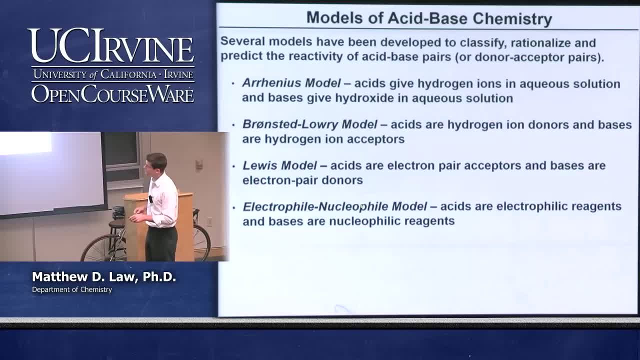 of the reactivity of the species that you're looking at: Electrophile, nucleophile. it's basically the same thing as the Lewis picture, But this is applied very commonly- this kind of language in organic chemistry. And then there are a number of acid-base concepts that 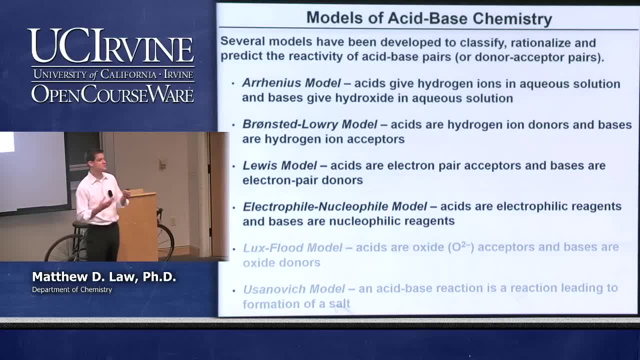 have not really stood the test of time or are very specific Right. so the Lux flood model, which is applied to geology and it looks at acids with relation to the oxide ion, And the Ossianovitch model, which is a very general model that basically hasn't really gained. 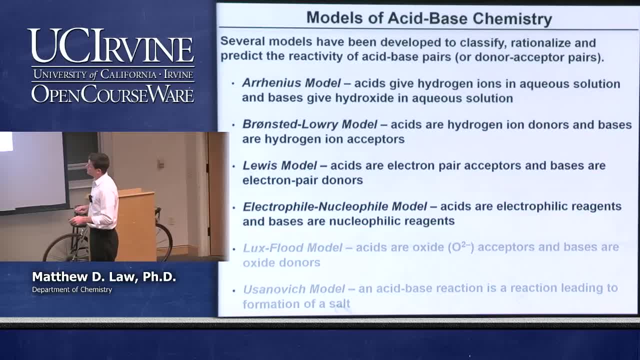 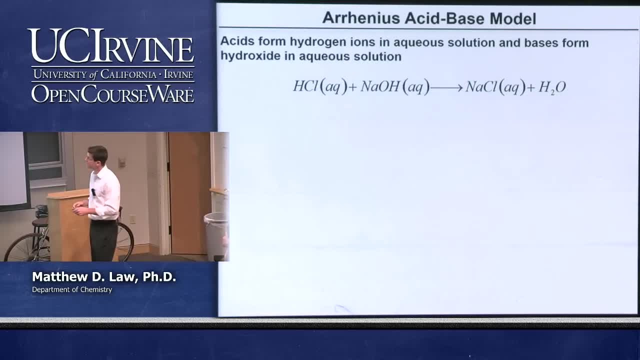 a lot of traction, And there are others too. Okay, so let's look very quickly at a review of Arrhenius and Lowry-Bronstedt and then we're going to get into the Lewis picture. So the Arrhenius acid-base model acids are hydrogen ions. provide hydrogen ions in aqueous. 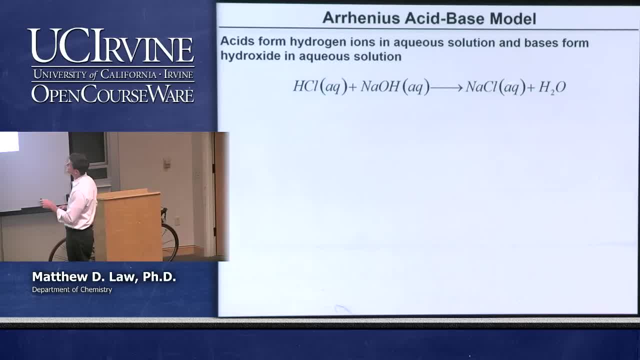 solution bases provide OH- in aqueous solution. Here is the prototypical acid-base reaction: Acid plus base, giving us a salt plus water. This is the way that it typically goes down: HCl, acid, sodium hydroxide base giving us. 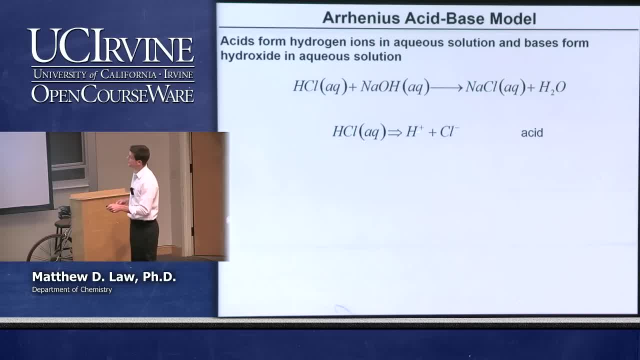 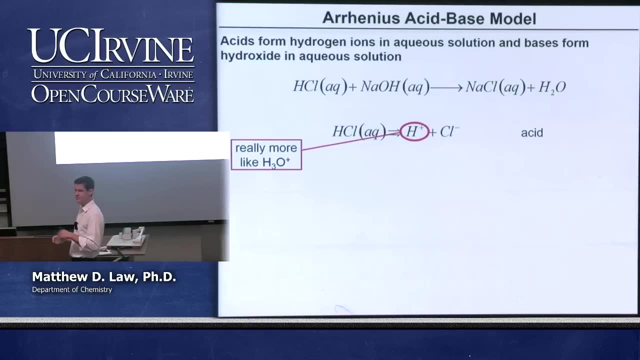 salt and water. The acid in the Arrhenius picture provides hydrogen ions. We know that really this is not proton. This is something more like hydronium ions. But even H3O plus of protonated water is not the most accurate way to portray this. Really it's a proton. 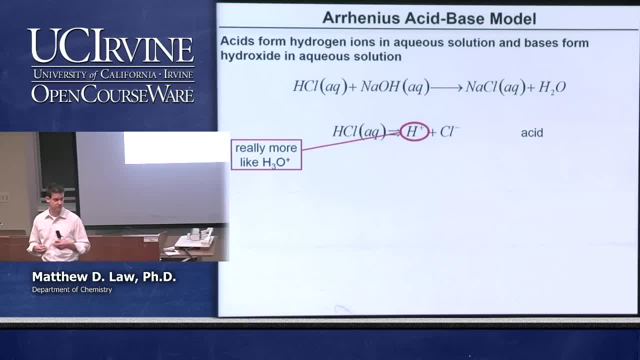 shared in a cluster of water molecules. So it might be a cluster of four water molecules with one proton hanging around. It's kind of an even more accurate way of describing it, But we'll go, of course, with the hydronium picture. So H3O plus is really what we're. 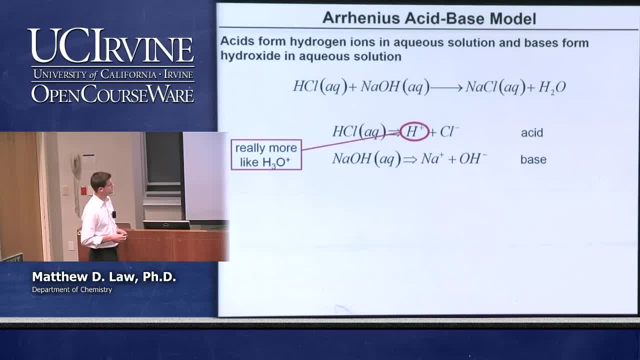 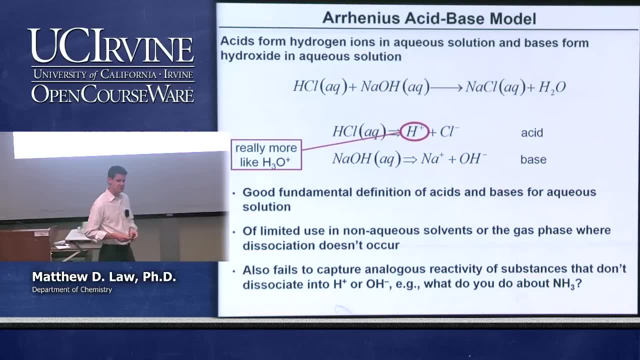 talking about here. The base provides OH- to solution. This is fine, right, It's a good picture for aqueous chemistry, but it has a lot of limitations. It's very specific, So it's of very- it's very limited use. 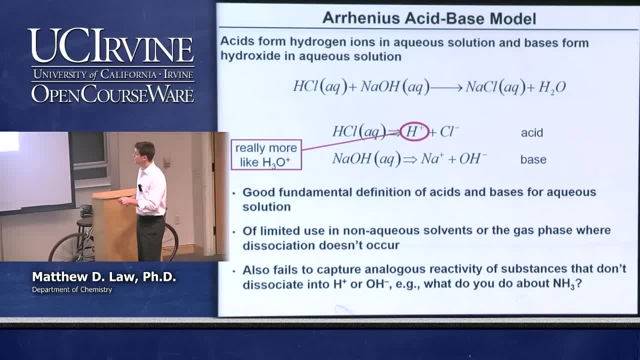 Non-aqueous situations, And it's also of limited use when we have substances that don't dissociate into these two species. So, for example, we know that ammonia has acid-based properties, but how do you describe ammonia in the Arrhenius picture? You really can't. 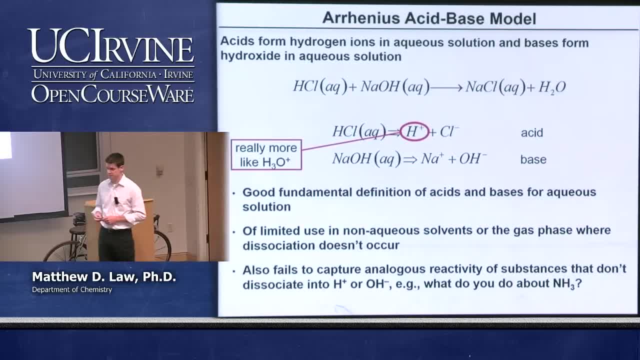 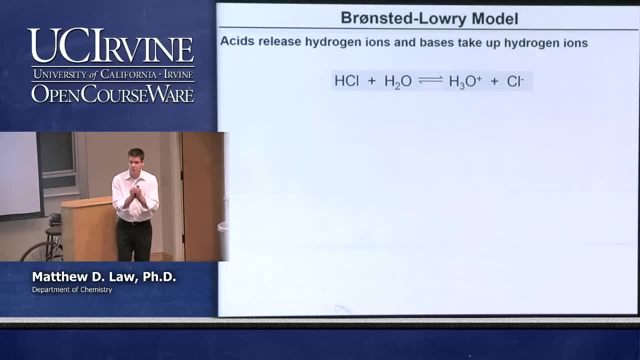 because it's not providing H plus or it's not providing OH- directly anyway. So that's the most specific definition that we currently kind of talk about these days. A more general definition is that it provides H2O. This is the Lowry-Bronsted picture. Here we have proton or hydrogen ion donors and acceptors. 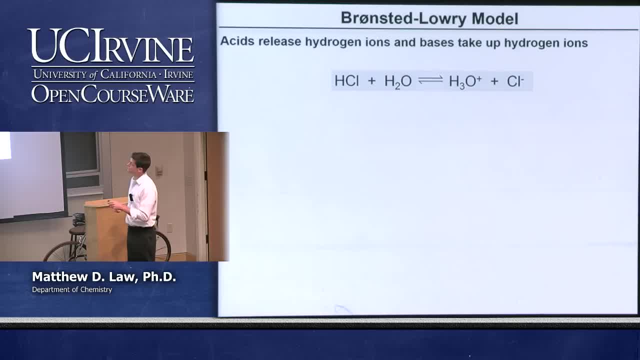 right. Here's a nice Lowry-Bronsted reaction: HCl plus water, giving us H3O plus plus Cl minus. And in the Lowry-Bronsted picture we always have the concept of kind of duality. We have conjugate pairs, We have acid-base pairs that are always on both sides of the equation. 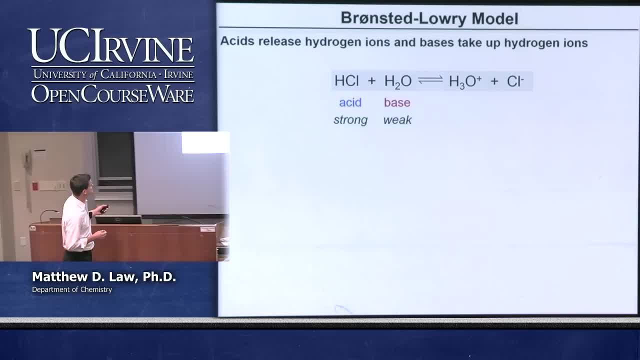 We have an acid and we have a base, So we can describe this as, of course, a strong acid HCl reacting with the weak base water, providing another acid in the base, in this case the weaker acid hydronium and the much weaker base chloride. So we have an acid-base. 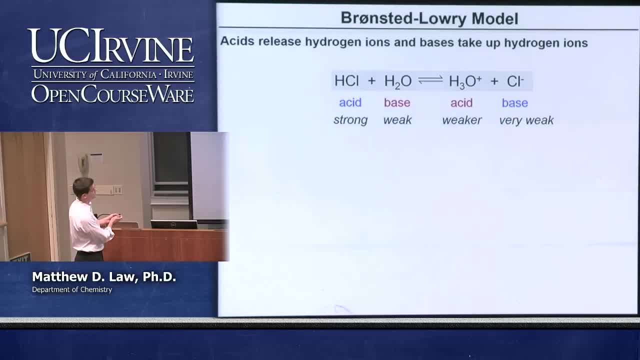 conjugate pair here that are interrelated by just the gain or loss of a proton. And we have a second acid-base conjugate pair here, again interrelated by the gain or loss of a proton. So we always have two conjugate base- acid-base pairs. We also always have 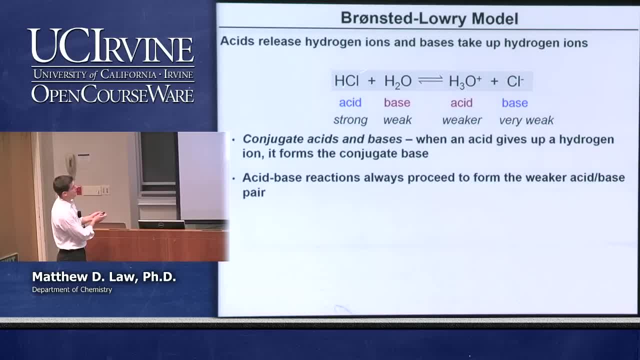 the reaction going in the direction where we go from the stronger acid-base couple to the weaker acid-base. This is the direction that equilibrium is going to lie In this particular case. we know just intuitively that when we put HCl in water, we're going. 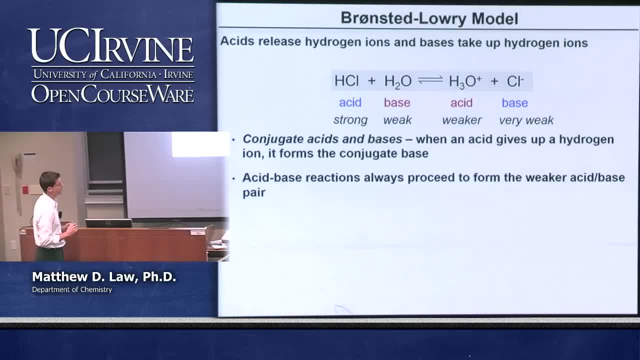 to generate all of this. The equilibrium lies very strongly on the right hand side And we can understand that in terms of the strengths of the acids in the bases. So we have a very strong acid producing a weaker acid and we have a weak base producing a very, very weak. 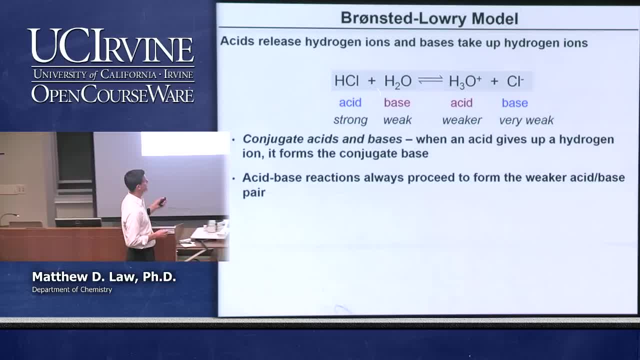 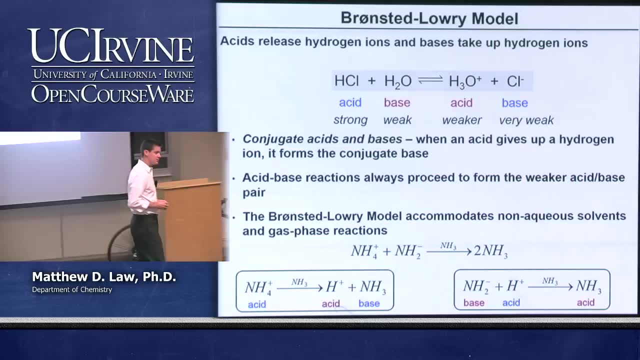 base, essentially, And so, because these are weaker than these, we have an equilibrium, in this case that lies on the right hand side. The nice thing about the Lowry Bronson picture, of course, is that we can apply it to situations that are not aqueous, So including solvents like ammonia, So we can have an ammonia we. 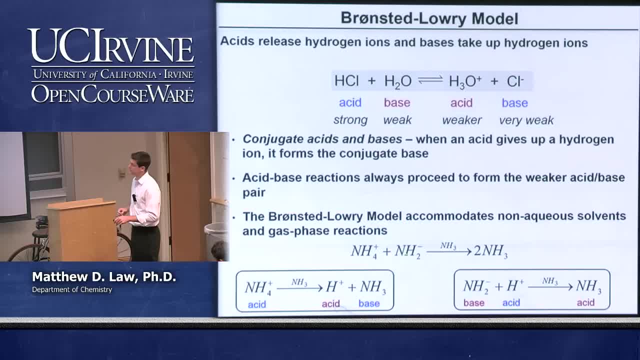 can have protonated ammonia and we can have deprotonated ammonia And having these two species. this would be your acid, this would be your base, producing two molecules of neutral ammonia in this case. So we can apply Lowry Bronson concepts to non-aqueous situations. 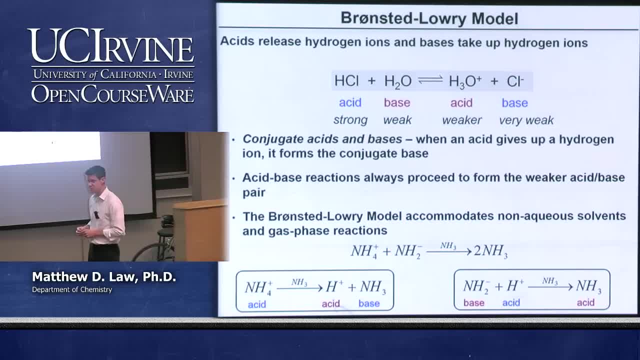 We can even apply Lowry Bronson concepts to gas phase reactions. right, You don't need a solvent at all. So you can, for example, have ammonia and HCl gas and you can get an acid based reaction that produces ammonium chloride, which would fall out of the air, of course. 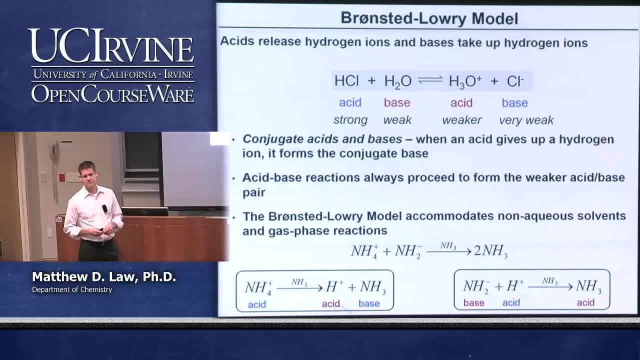 as a powder. That's a way that we can understand acid based reactivity in the absence of a solvent. Okay, So that's the deproton donor, proton acceptor kind of picture. This just expands on this reaction here, Always acid giving us. you know, conjugate acid base pairs in every case. 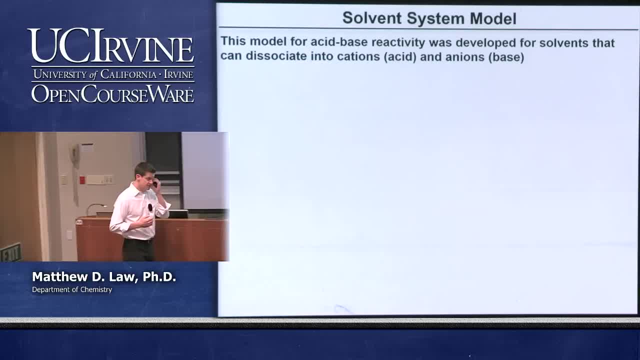 Okay, An expansion on the Lowry Bronson concept that we kind of highlighted there at the end when we talked about ammonia is that we can look in different solvents- right, It doesn't have to be water- And so we can develop something called a solvent system picture or solvent. 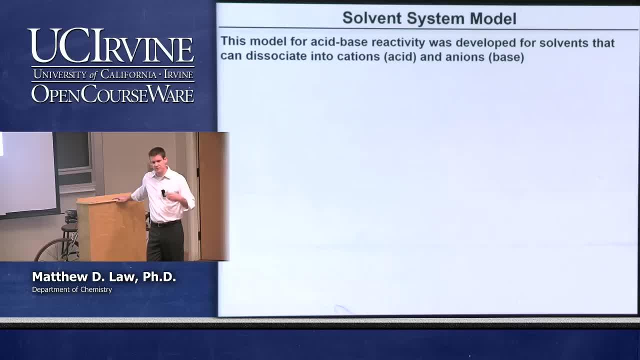 system model, And this accounts for acid based reactivity in the Lowry Bronson picture as well as in the Lewis picture. Okay, For solvents that can dissociate into cations and anions, Okay, A lots of solvents have a tendency to dissociate, at least to a very, very minor. 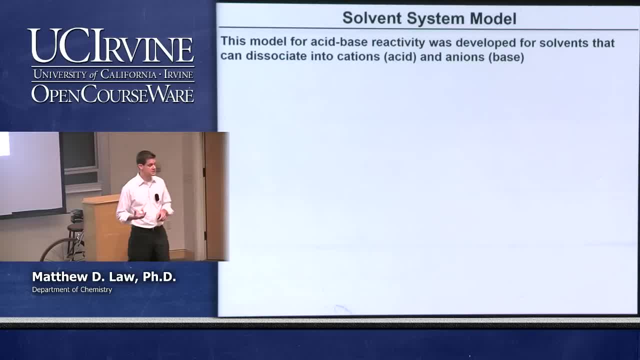 degree into cations and anions in solution. The normal example for this, of course, is water itself. So we have auto ionization of water, where one of the water molecules acts as a acid, the other as a base, and we produce H3O plus and OH minus. We ionize. 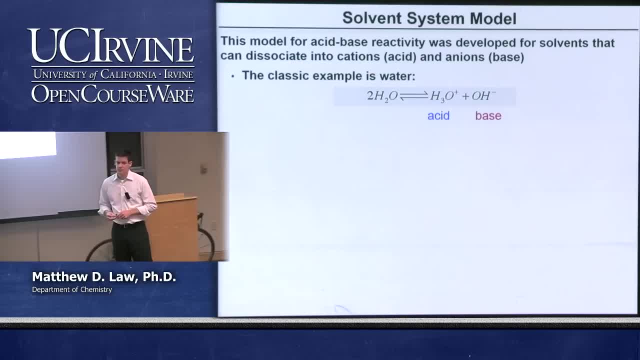 the two molecules into a cation and an anion And of course this determines a lot of the properties, the acid-base properties of water. It sets the strongest acid that's possible in water and it sets the strongest base that's possible in water. 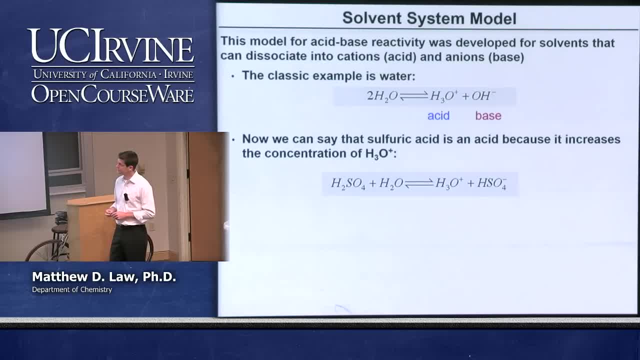 Well, lots of other solvents do the same thing to varying degrees. So, with the solvent system picture, what we can do is we can interpret the cations as the acids and the anions as the base, And so anything that produces a cation would be considered acid-forming or an acidic kind of species. 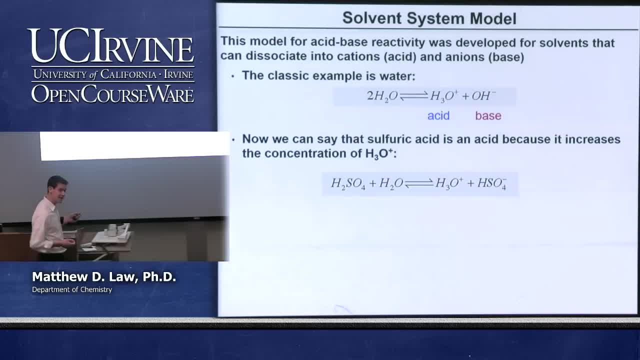 And anything that produces an anion would be a basic species. So in that kind of thinking we can think of H2SO4 as being acidic because it produces the cation in the autoionization picture. The cation then is the acid, so in a sense is the H2SO4.. 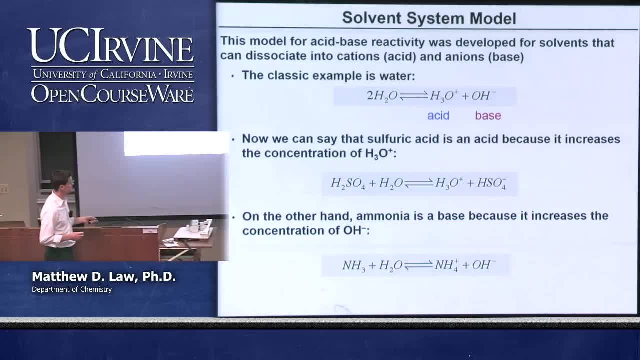 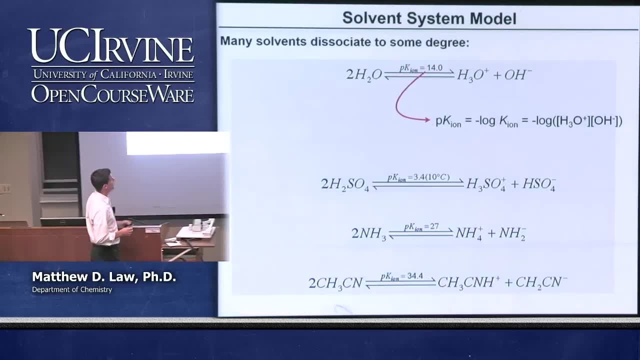 Same thing with ammonia. We can think of ammonia as a base, because what does it result in? Oh, It results in the anion in the solvent that we're talking about, And so we can do this with water. We can do this with lots of other solvents as well. 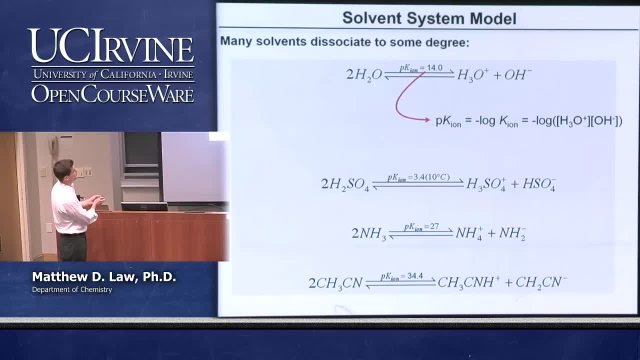 And this is just a list of a few. You'll probably remember that the autoionization has a Ka or a Kw of 10 to the minus 14.. And so the pKw, in this case what we just call the pK- of ionization. 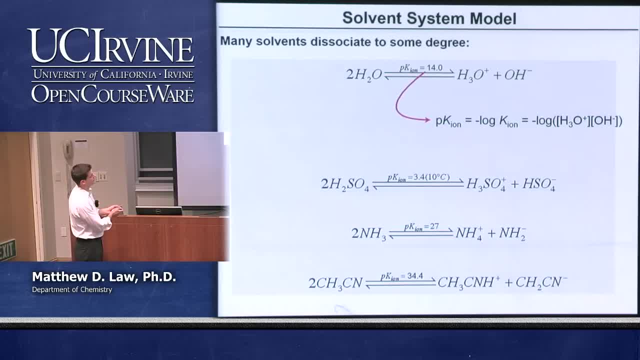 so this reaction, this equilibrium constant negative log of that gives us a value of 14.0.. So that's related, of course, to the concentrations of the cation and the anion in solution at equilibrium. Well, we have the same sort of reactions, these autoionization reactions for sulfuric acid. 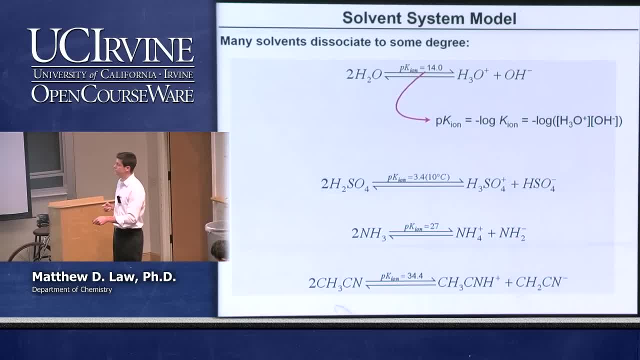 We have them for ammonia, We have them for acetonitrile and many, many others. You can see that in the case of sulfuric acid, we have a pretty low pK ionization And that means that we're going to have fairly large concentrations of these two species in solution. 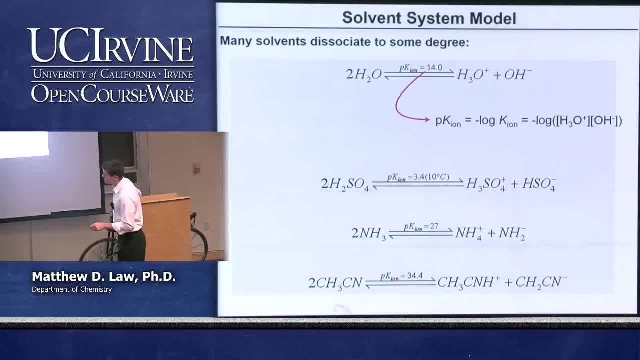 Right. If you look down at acetonitrile, the pK of ionization is very, very large, which means that the concentrations of the cation and the anion are very, very, very small, of course, but not zero. 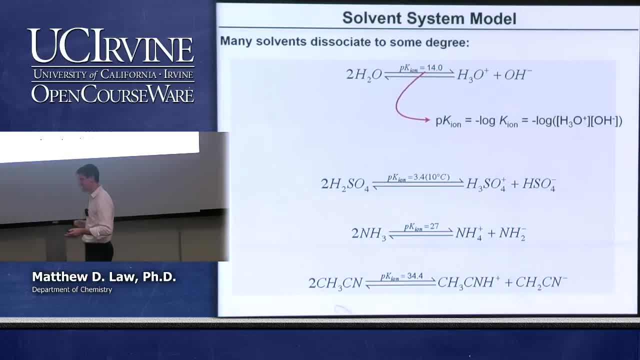 And so you can have the same sort of analogous chemistry as you know, the normal Bronsted picture in water. applied to these other solvents, All the values for the Ka's and the Kb's will of course, depend on the solvent very strongly. 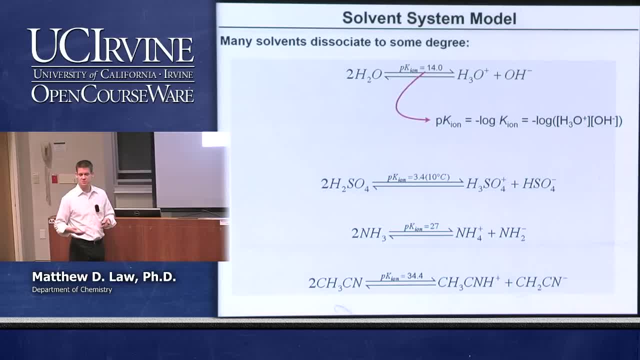 So what we know about acetone is that it's a very strong solvent, Right Right, Right Right. So the amount of acids and bases in water doesn't necessarily transfer, certainly doesn't transfer quantitatively to those reactions occurring in ammonia. 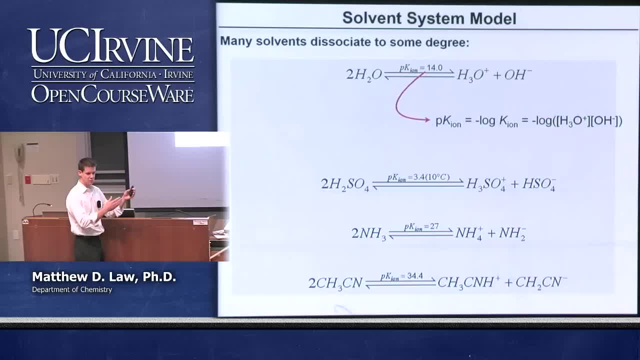 Right, There are those reactions occurring in acetonitrile, But we can develop an equivalent scheme in those other solvents And people have done this. So these are all shown. for you know protonation and deprotonation, So we have a cation and anion that's exchanged a proton. 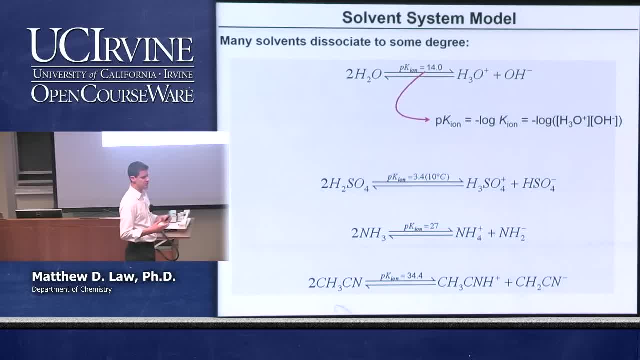 But it doesn't have to be ionization from proton exchange, It can be more general, So we can have, you know, non-protic situations where we have dissociation occurring, and this leads us kind of to the Lewis picture. So we can describe that sort of stuff in solvents that are aprotic. 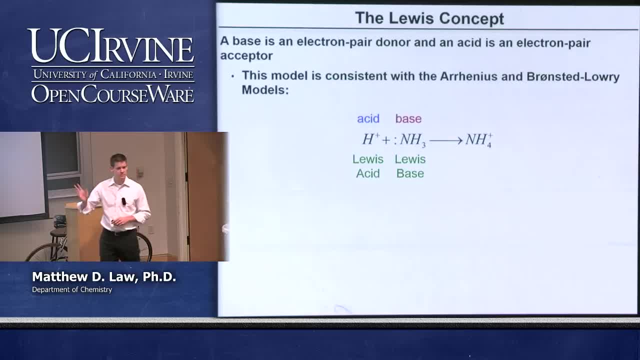 Okay, any questions about the hopefully fairly well-known and very familiar feeling Arrhenius and Lowry-Bronsted pictures. Okay, so now let's talk about the Lewis picture. Again, you've taken organic chemistry, so you've probably been pummeled with Lewis acid-base chemistry a little bit. 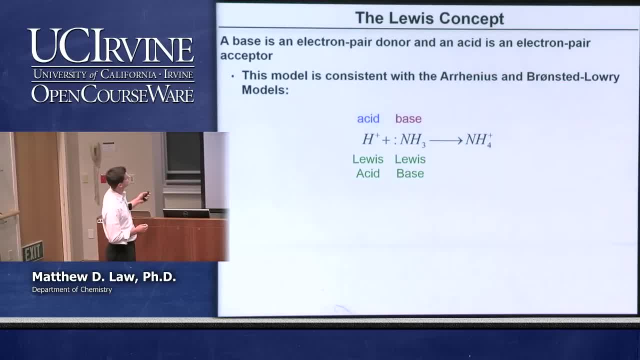 We're going to take a different approach. Lewis concept fairly straightforward and it's a more general interpretation of acid-base chemistry. So base is an electron pair donor and acid is an electron pair acceptor. And the Lewis picture is consistent with the Lowry-Bronsted and the Arrhenius pictures. 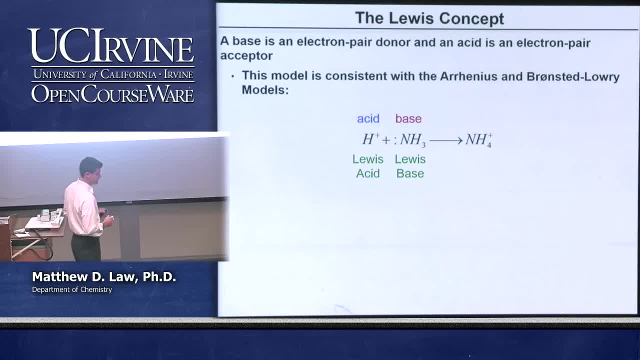 So we can think of A Bronsted acid, okay, as also being an example, one example of many different types of Lewis acids, Because the Bronsted is, you know this, proton or H3O+. it's going to accept an electron pair from a base. 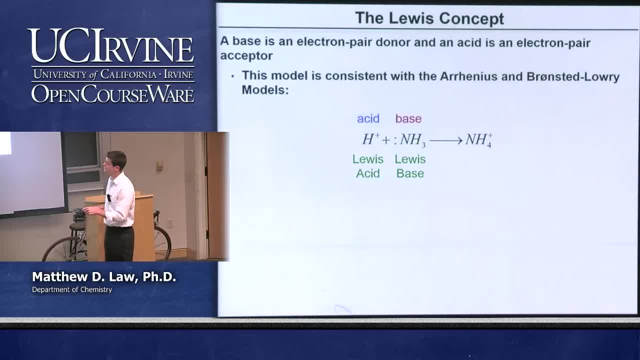 In this case, in our reaction. here we have our Lewis base being ammonia, Okay, and you can form that ammonium ion. So this is an example of Lewis acid accepting an electron pair, Lewis base donating an electron pair to form what we would call an adduct. 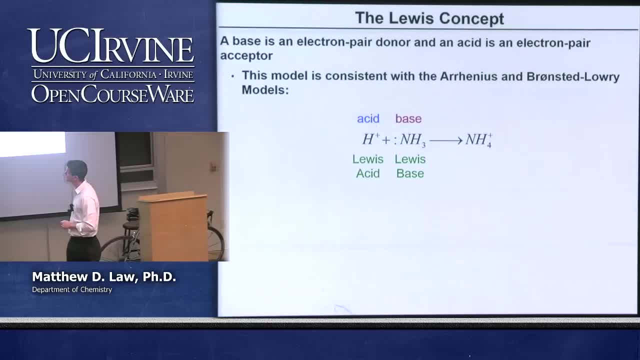 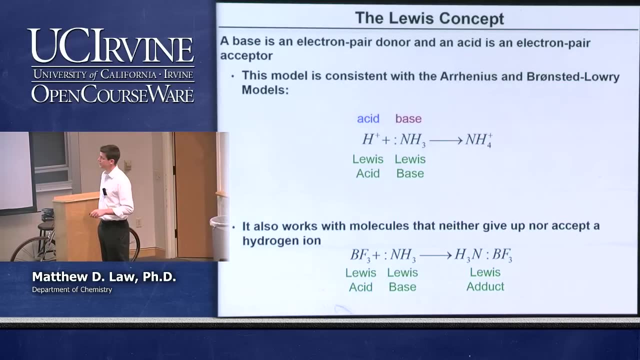 Okay, Lewis acid Base adduct. So the Bronsted picture is a subset of Lewis chemistry. Okay, because we can have lots of different kinds of Lewis acids that aren't necessarily just protons. One example of a molecule reaction that doesn't involve hydrogen ions at all is the most classic Lewis acid-base reaction. 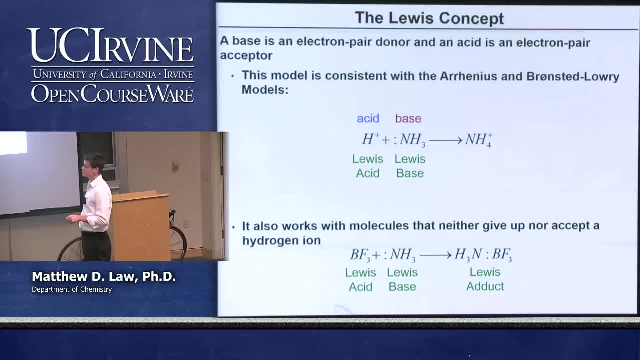 BF3, Lewis acid, Lewis base ammonia forming a Lewis adduct, Okay, Electron pair being donated to the BF3 molecule to form this new molecule, this Lewis adduct. So we have Lewis acid-base chemistry occurring without protons. 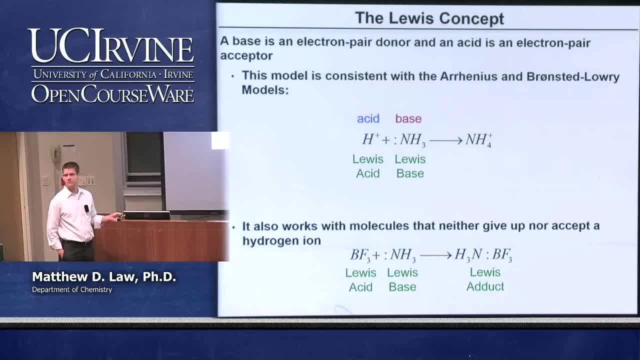 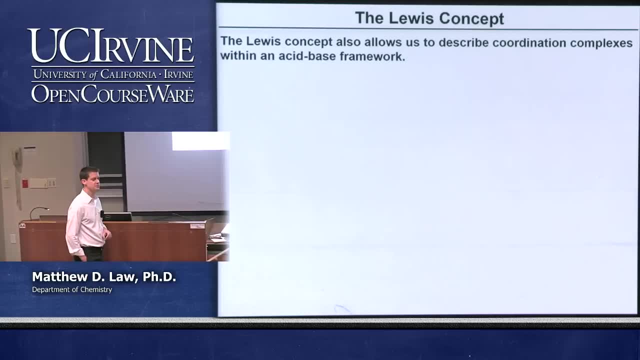 Okay, Any questions? Okay, All right. So the Lewis concept is quite powerful and broad and directly applicable to lots of reactions in organic chemistry. That's why we're going to focus on it. One of the most important reactions in inorganic chemistry- that is, a direct application of Lewis acid-base concept- is the formation of coordination compounds. 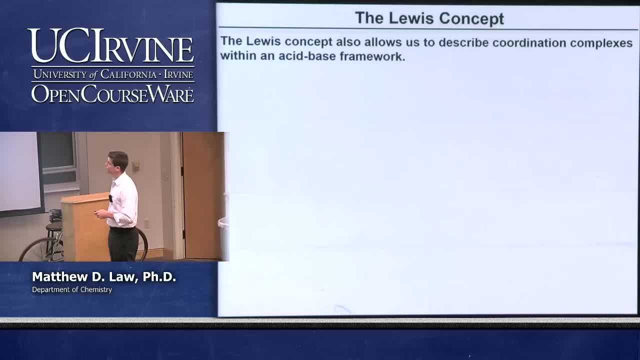 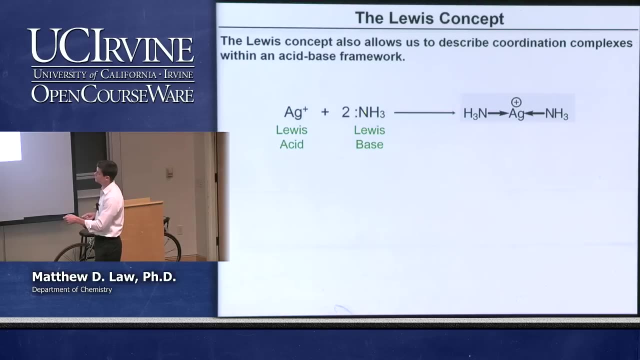 So metal complexes. Okay, We can almost always understand the formation of a metal complex. This is where we have one or more metal atoms interacting with ligands. Okay, In terms of the Lewis acid-base picture. So here's a reaction of silver plus plus two ammonia, giving us this metal complex. 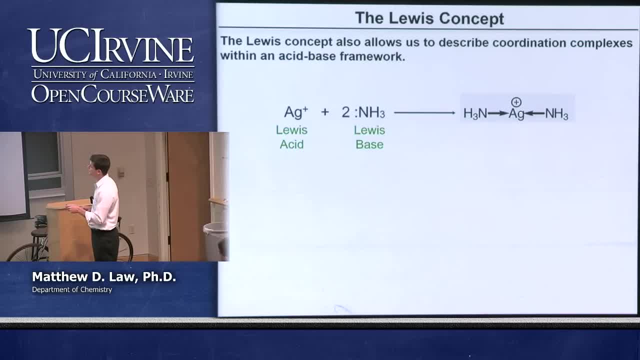 Okay, We have this diamine, silver plus, Okay, Silver one. The silver in this case is electron efficient. It's going to act as a Lewis acid. It's going to accept electron density from the Lewis base, which is again our example of ammonia, and form this metal complex. 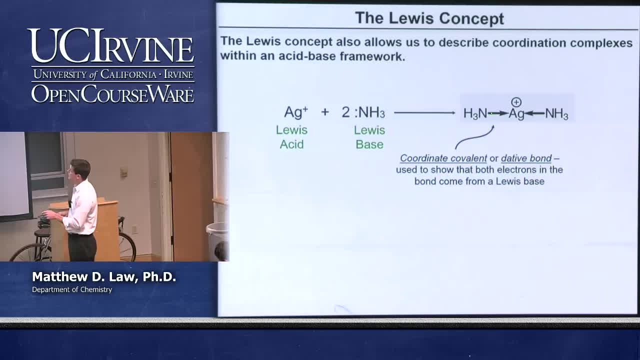 Okay, The way I've drawn these bonds is a little bit strange with these arrows. Okay, This is meant to indicate that both of the electrons from the bond are coming from the Lewis base. Okay, So this kind of bond from ligands, you know, Lewis base, to a central metal atom is called a coordinate covalence or a dative bond. 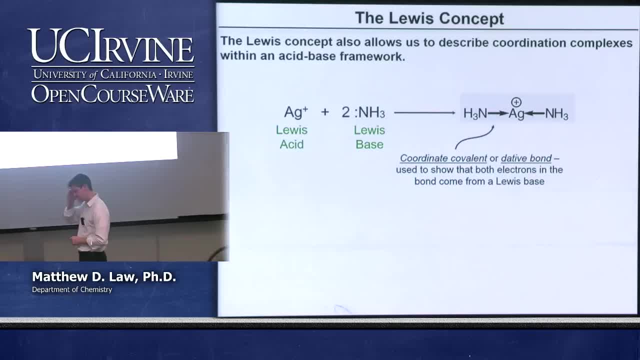 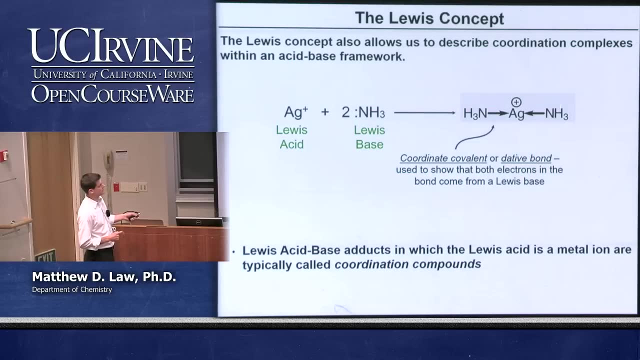 And sometimes you see it drawn with arrows like that. Usually the arrows are omitted, but that's just to remind us from where the electron density came. Okay, So these adducts here. we can describe this as a coordination compound or an adduct. 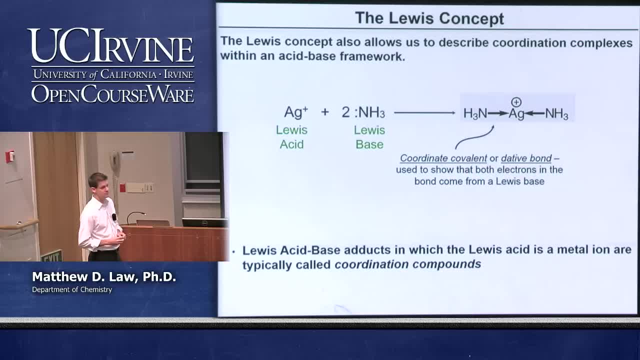 Okay, Lewis base adducts in which the Lewis acid is a metal and Lewis base is anything. Okay- Are often called coordination compounds if we're talking about neutral species, or kind of coordination complexes if we're talking about charged species. And so the latter part of this class, basically the last third of the entire class, is going to be about coordination compounds and complexes. 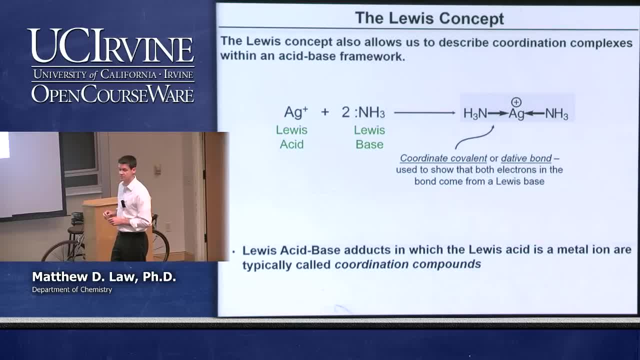 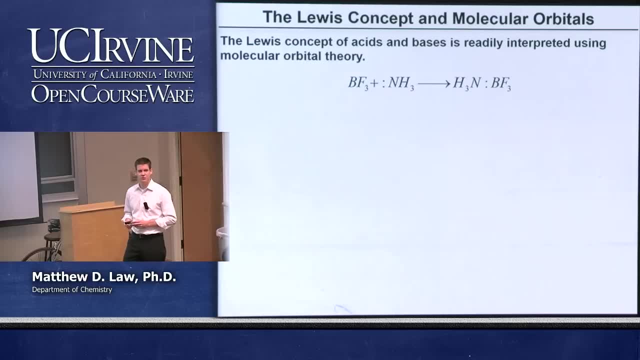 So we can always understand their formation in terms of the Lewis acid base picture. Okay, Let's apply now what we've learned about molecular orbital theory to understand the driving force and kind of the structure and what's going on in general with Lewis acid base adduct formation. 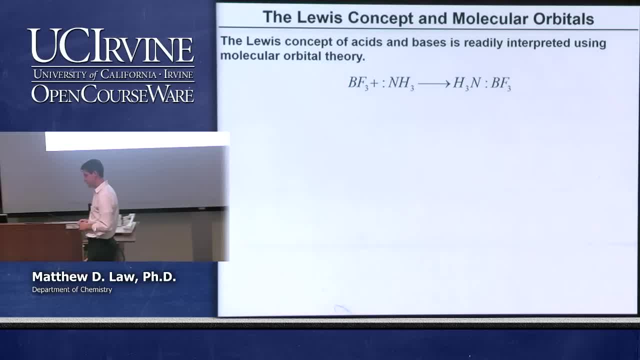 So we can easily interpret the Lewis concept of acids and bases with molecular orbital theory. What we can do is we can look at our prototypical example here- BF3 plus NH3. And understand what's going on. Okay, We can identify this right away as the Lewis acid and this is the Lewis base. 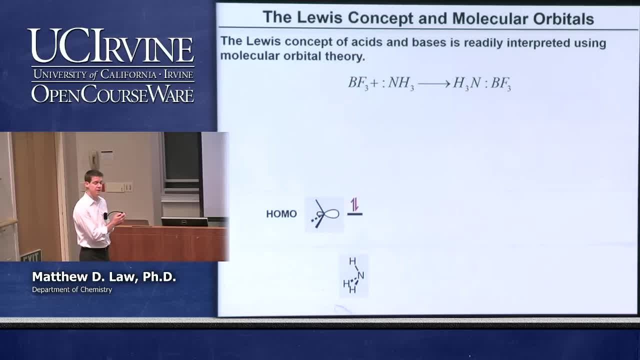 Okay, We know that. Let's draw an MO diagram showing the bonding that's going to happen in the adduct. Okay, When we form this boron-nitrogen sigma type bond, If you remember, from ammonia, the molecular orbital diagram from ammonia has a HOMO, where most of the electron density is a non-bonding orbital located on the nitrogen. 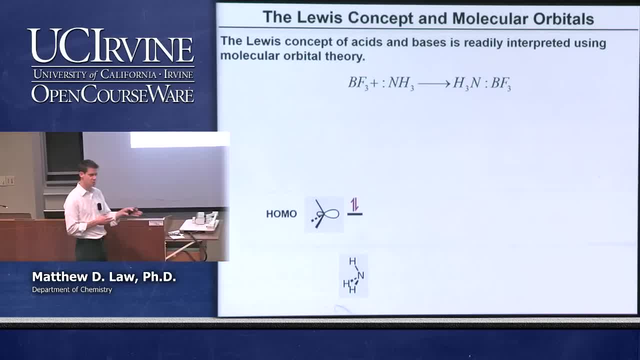 Okay, Going right between the three hydrogens and pointing away from the nitrogen. Okay, And pointing away from those hydrogens. That's the lone pair on nitrogen, Okay, In the Lewis dot picture. So that is the highest occupied molecular orbital of the base. Okay, And of course that's where the electrons are going to come from, to make the bond, the coordinate covalent bond or the dative bond, to make the adduct. On the other side of the diagram, we have BF3, which we also developed, the molecular orbital diagram of. 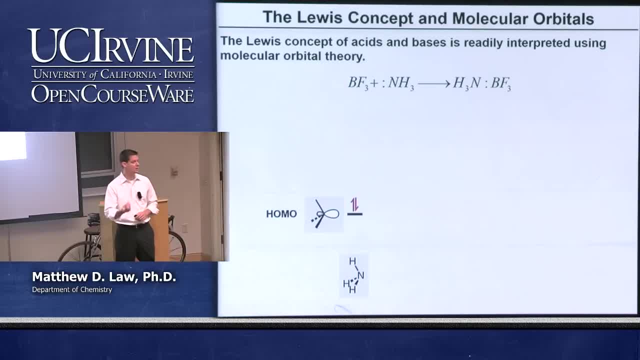 And you may or may not remember that the LUMO for BF3 is a pi anti-bonding LUMO. Okay, And we also developed an anti-bonding LUMO for it And we also developed a molecular orbital diagram of it. 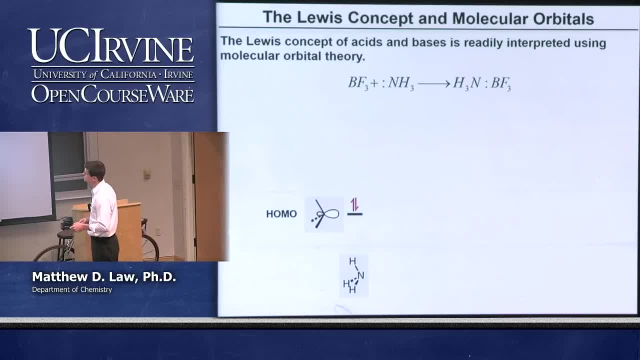 Okay, And you may or may not remember that the LUMO for BF3 is a pi, anti-bonding LUMO. Okay, On the other side of the diagram, we have BF3, which we also developed the molecular orbital diagram of. 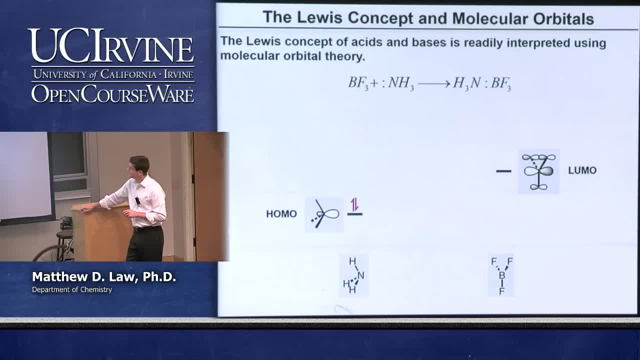 And you may or may not remember that the LUMO for BF3 is a pi- anti-bonding LUMO, where most of the lobe is on the central atom, the boron. Okay, And you can see right away that you've got some nice, proper symmetry there for making. 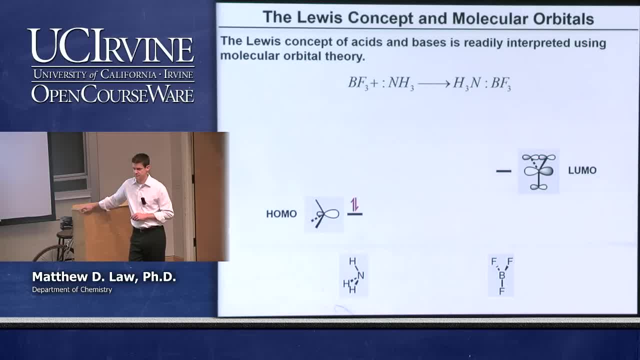 a sigma type bond between the boron and the nitrogen. Okay, Okay, It's LUMO, So it's unoccupied, which means that we have no electrons present in that orbital. Now, what we're going to do is we're going to make our bonds to form our adduct. 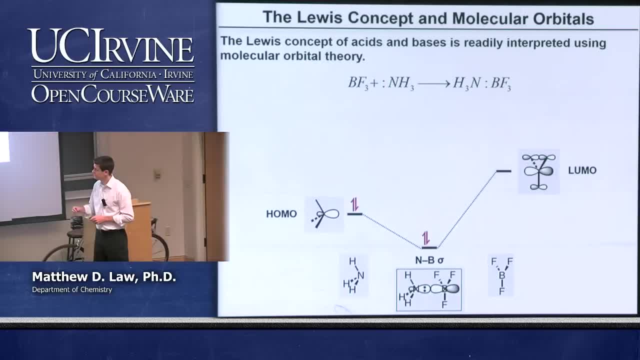 We're going to make a sigma bond and we're going to make a sigma antibond. The sigma bond looks something like this, where I've just kind of simplified some of the orbital sketch. here You've got, of course, a nice sigma bond where the two electrons are coming in from nitrogen. 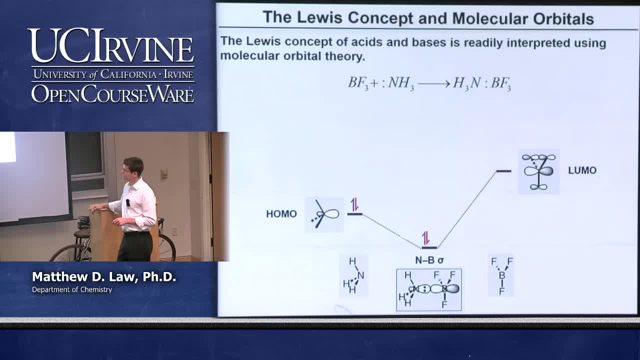 Those two electrons from nitrogen are decreased, stabilized in energy when the bond is formed. And then, of course, we have an antibond sigma style as well, where we've just, in this case, flipped the polarity of the boron-based orbital. 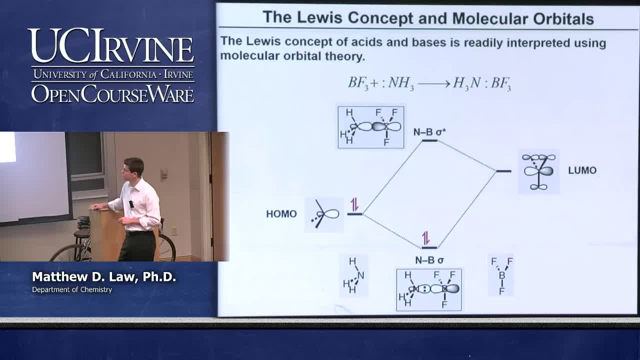 So we have no electron density here and we have an antibond sigma star orbital That's not filled, of course, because we only have two electrons in the frontier orbitals for the molecule. The driving force for adduct formation is just this. 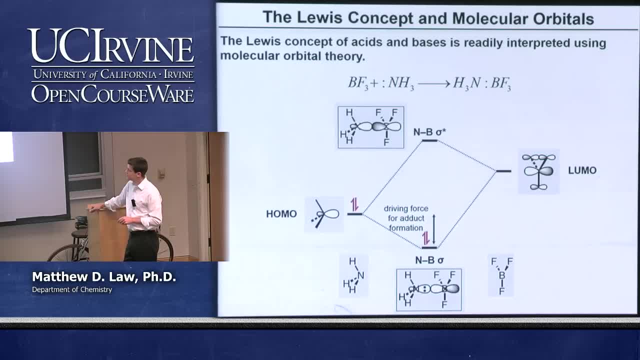 More or less So. the driving force is the decrease in the energy, the stabilization in energy of this lone pair of electrons, here because it falls into a bonding orbital, And so the MO picture gives us a quite nice and fairly straightforward understanding about how the adduct forms and why the adduct forms. 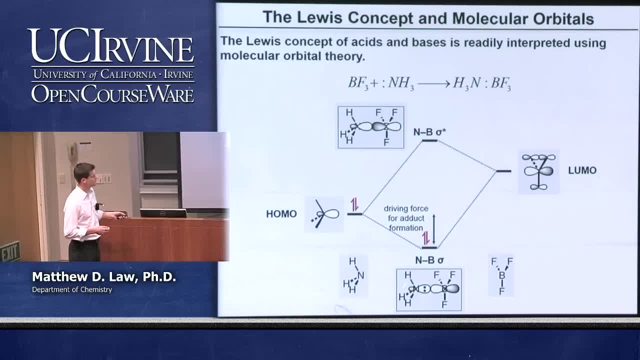 You probably have noticed down here that I haven't properly drawn the molecule. After the bonding has happened, of course the boron goes into a pseudo-tetrahedral situation. It's not planar anymore. But of course, as the molecule forms its point, group changes. 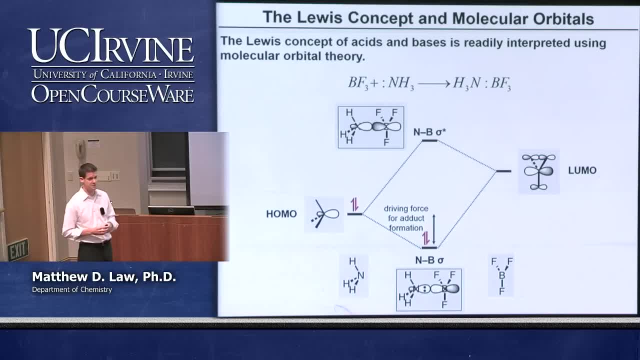 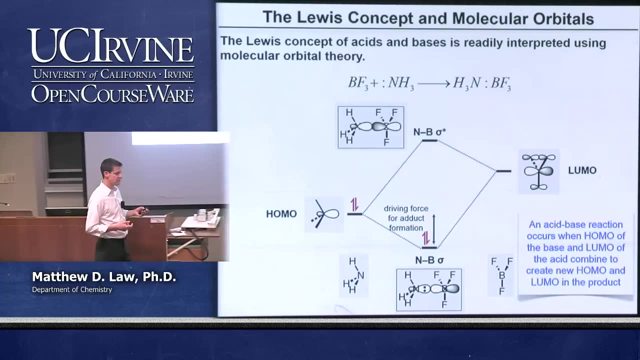 There's differences in bond lengths, differences in bond angles and so forth, But the general idea is that we form a sigma bond and a sigma antibond and we fill the bonding orbital. So what can we say in terms of molecular orbital theory about Lewis acid-base chemistry? 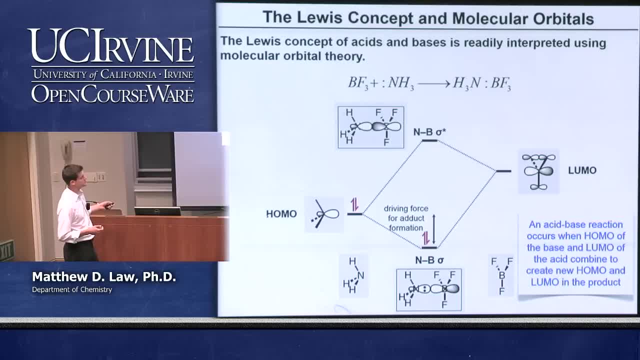 We have an acid-base reaction when the HOMO of the base and the LUMO of the acid have the right symmetry and the right energy to interact and form a bond and an antibond. So we're always looking at the position of the HOMO versus the position of the LUMO for the base and for the acid. 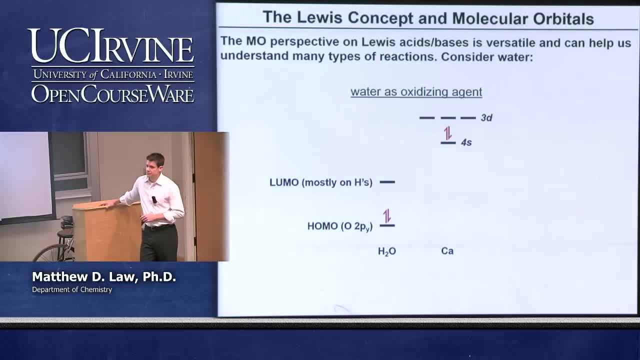 Okay Now, just like in the Lowry-Bronsted picture, we know that certain species are amphoteric. They can react as either acids or bases, And water is a great example of one of these species. It can accept a proton or it can donate a proton. 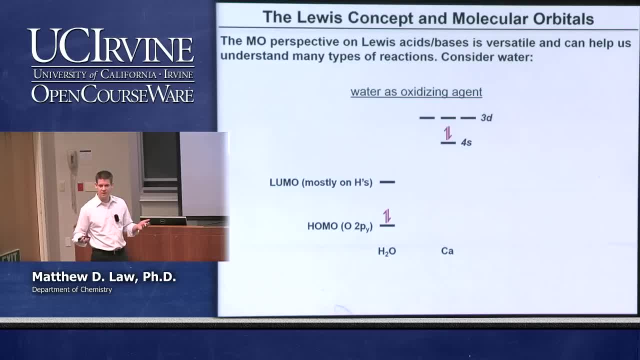 So it can act as either a base or an acid. It's the same thing for lots of Lewis- almost all Lewis acids and bases. Your behavior as a Lewis species depends on what you're reacting with. So you may in one circumstance act as a Lewis acid, but in another circumstance act as a Lewis base. 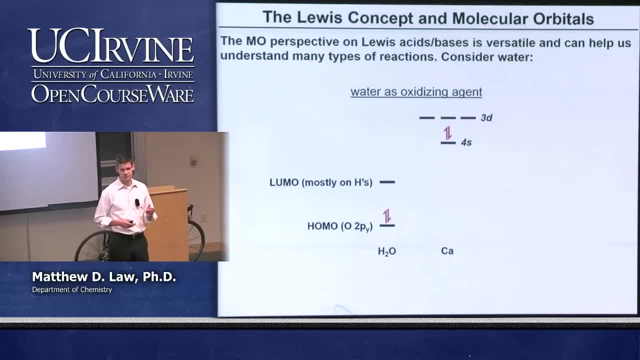 And water is again a nice example of this kind of very versatile chemistry And we can understand sort of the spectrum of reactivity for these sorts of compounds, these sorts of materials, looking at a simple molecular orbital picture. Okay, So the molecular orbital perspective. 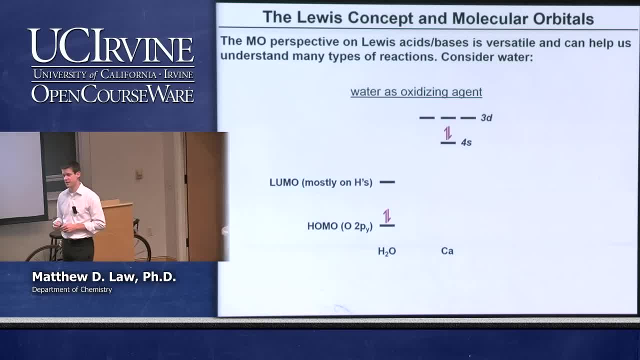 Versatile and can help us understand lots of different classes of reactions, Including all the way to redox reactions, So we can rationalize redox reactions in terms of MO theory. So let's do this by looking at water and comparing water's reactivity with a number of other partners. 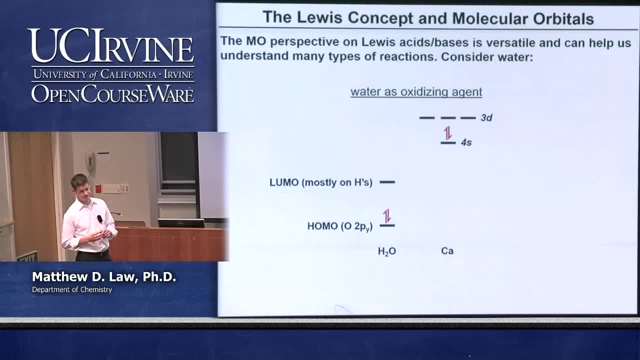 Let's start first by looking at water as an oxidizing agent. Here's water's HOMO-LUMO, the frontier orbitals for water. Remember that the HOMO right It is the non-bonding oxygen-centered 2P-Y orbital, in this case. 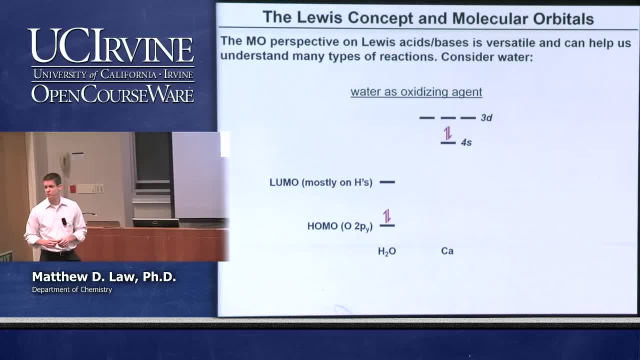 We have two electrons there: The LUMO. we didn't really focus on what the LUMO looks like in water, but it's based primarily on the hydrogens, Anti-bonding and it's based primarily on the hydrogens And this is the you know, let's just say, schematic energy of these orbitals. 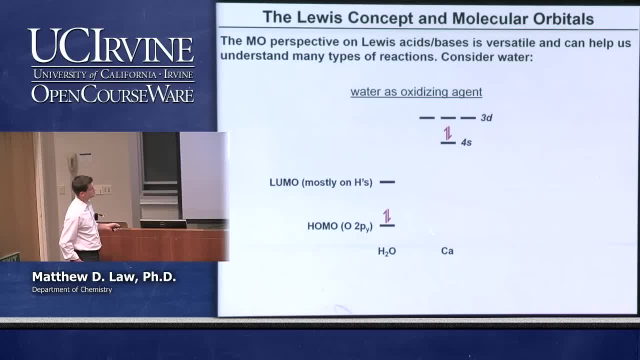 If we react water with a species that comes in that has electrons located much higher in energy. For example, calcium coming in, Calcium metal has two electrons in the 4S orbital. Those are quite higher, much higher than the LUMO for water and certainly much higher than the HOMO of water. 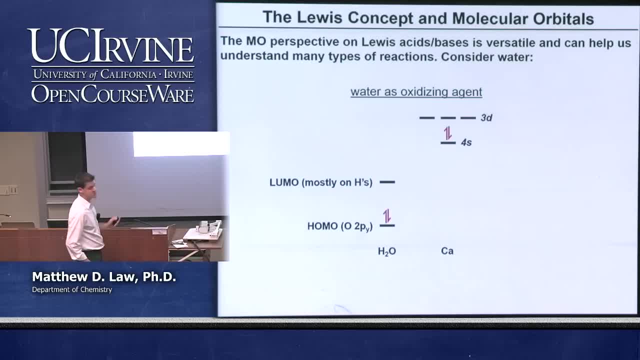 We see here that we have a large driving force for those electrons to jump to water essentially, And so, because of this very large energy difference, we can consider this to be, you know, many electron volts of driving force. perhaps The tendency is not going to be to make a bond and anti-bond but to transfer the electrons. 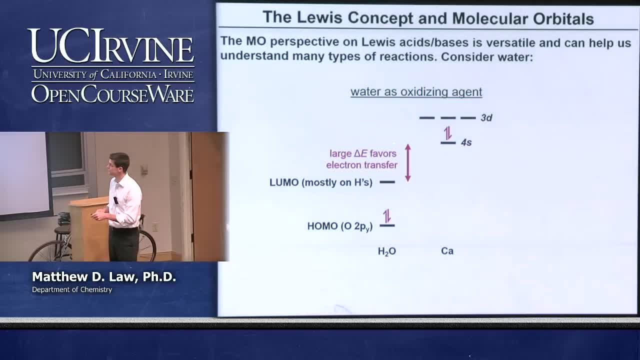 The electrons are going to be transferred from one species to another because of this very, very large energy difference between the molecular orbitals on the individual constituents. And so in this kind of case, what's going to happen is that water is going to oxidize calcium zero to calcium two. 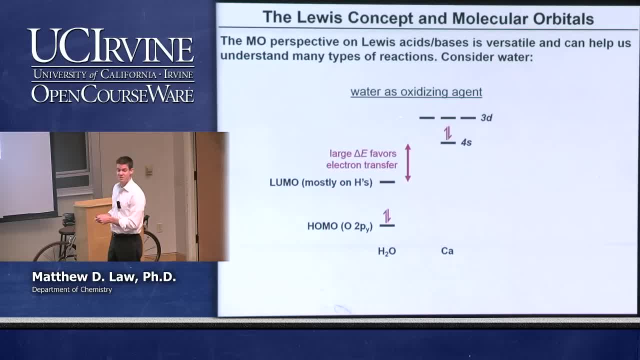 Those two electrons you can imagine momentarily lie on the LUMO, Okay, Forming water, two minus Or something like this. Okay, But of course that's not a stable situation, and what water is going to do is it's going to decompose. 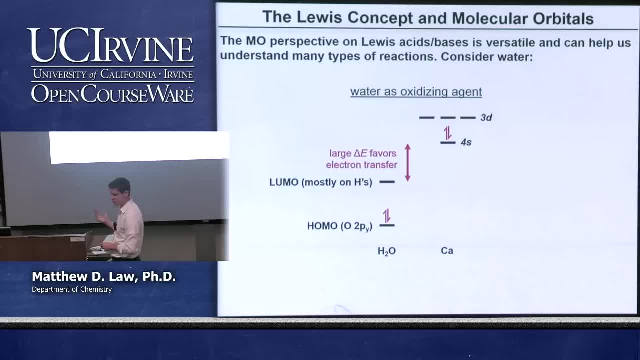 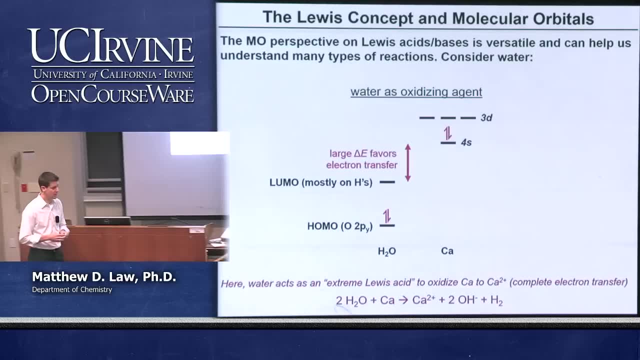 And you're going to make, because we've oxidized calcium. you're going to make something that's reduced on water, Or you're going to decompose water into something that's reduced, And so the reaction that you end up having here is you have waters plus calcium, oxidizing the calcium because of this electron transfer. 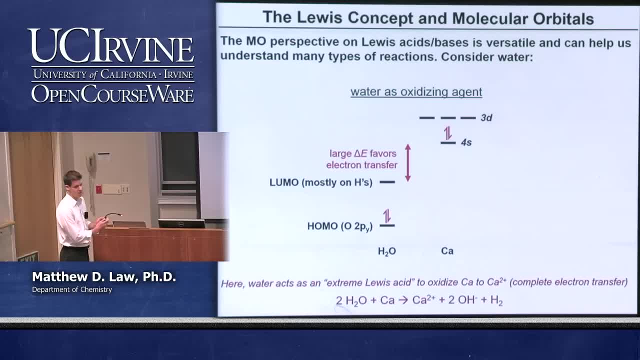 And you're reducing then water to hydrogen and to OH minus. Okay, So water breaks apart And we can understand this sort of reaction. as an example where we have an extreme Lewis acid- Okay, Where water is the Lewis acid, of course. 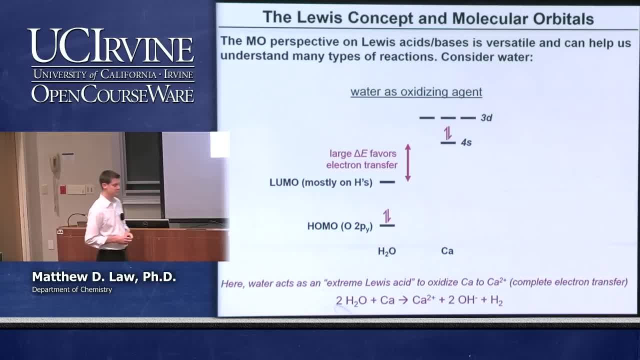 Okay, The electron pair acceptor, And it's oxidizing something from, in this case, zero to plus two oxidation state. Yeah, What's the delta E that would be required for it to be characterized as extreme? Yeah, It is totally vague, right. 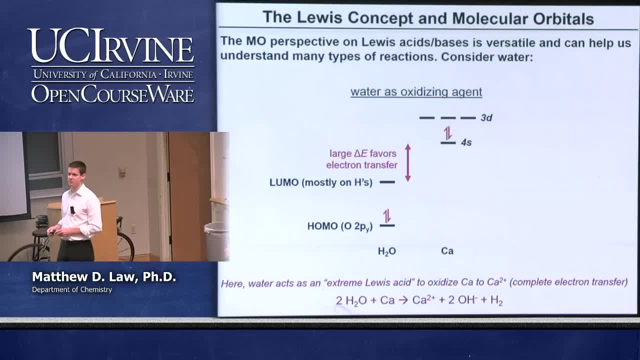 It just depends. Yeah, So I don't have a rule of thumb even for that energy difference. Yeah, And this is you know. let me emphasize: it's a way to rationalize qualitatively the chemistry that's observed in terms of the MO picture and the Lewis acid base picture. 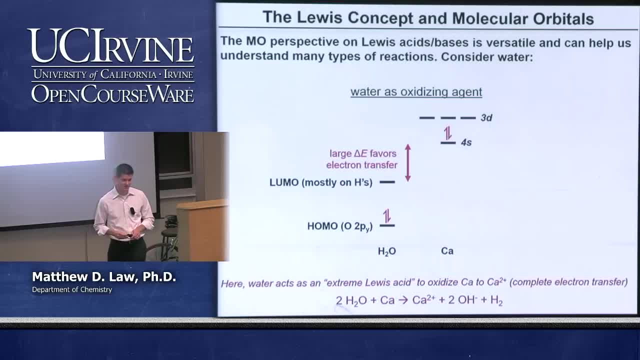 So in many cases you might expect, with kind of a smaller energy difference, to have some shared electron density, But still you have a redox reaction happen, Yeah. So like all chemistry, right, the world is messy, Right, And what we're trying to do is understand, with you know, put reactions in boxes and try to understand qualitatively what's happening. 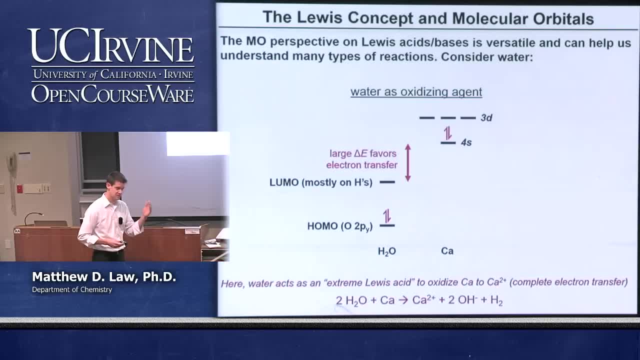 It's very difficult to do it in a way that is right most of the time, a lot of the time, all of the time, Yeah, It's tough to do that. So this gives us again chemical sets, Right Chemical intuition. 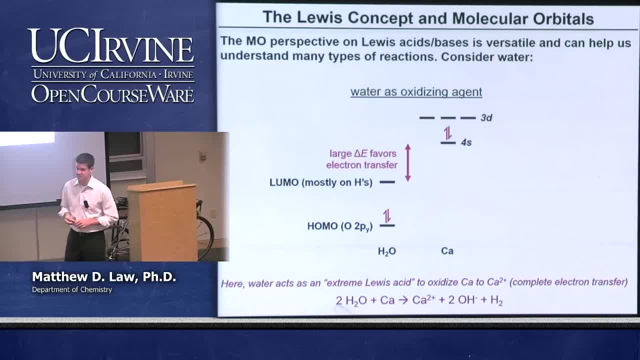 And some machinery to understand what to expect. Okay, Any other questions about water acting as an extreme Lewis acid that causes a redox reaction instead of adduct formation? Okay, So now what we're going to do is we're just going to change the species that water is interacting with. 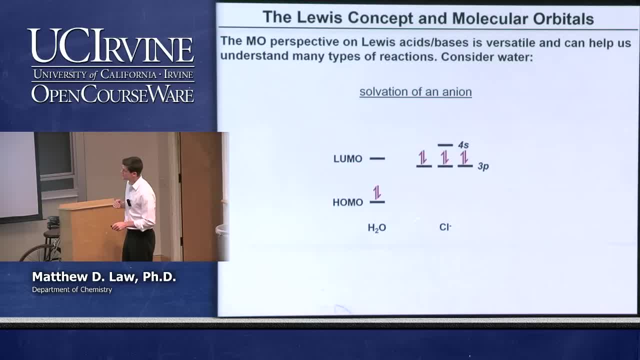 Let's decrease the energy difference a little bit. Okay, In this case, let's react water. put water in the presence of chloride ion. Okay, In this case: chloride ion, the homo, here is the three P's. Okay, Again unchanged for water. 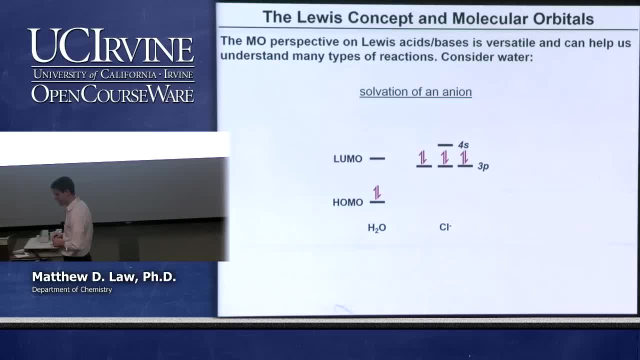 And the energy difference now is much smaller than it was, And you can have now a situation where you have the Lewis base interacting with water, again as a Lewis acid, but in this case forming an adduct, rather than having some sort of hard electron transfer. 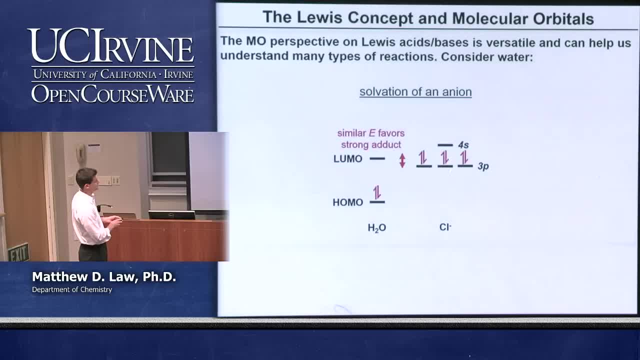 So we have a smaller energy difference now between the Lewis base homo And the Lewis acid lumo, And what you're going to have in a situation like this is just solvation of the chlorides. You're going to make an adduct. you can imagine, with some number of waters surrounding a chloride to form a chloride that's hydrated by n number of waters. 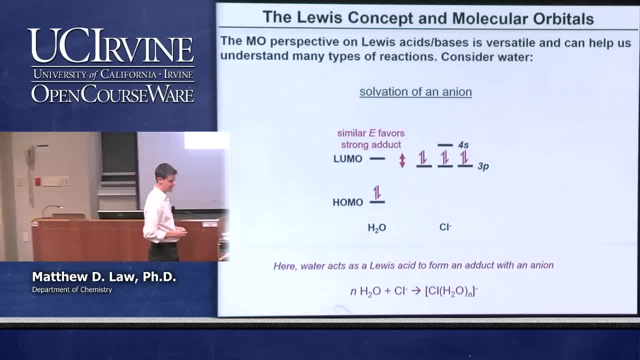 Where n might be four, Might be more than that, Four, six, something like this. Okay, So in this case the driving force for electron transfer is a lot smaller. That's one way we can rationalize that We're not going to have strong electron transfer. 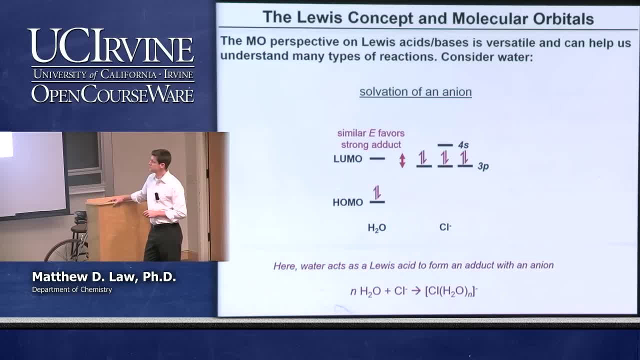 We also have, you know, interaction with an anion here, So chloride being quite stable, Happy where it is. So we're going to have bonding and anti-bonding between these one of these P orbitals and the lumo. 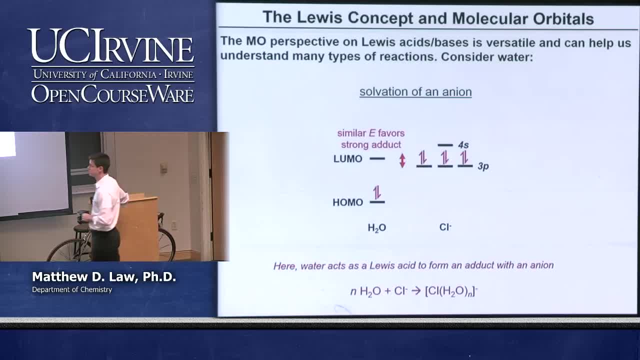 Okay, From each of the different waters coming in. Okay, Yeah, So the? n depends on several things. One of the things is size, So how many waters can fit around? the chloride is one important consideration. Yeah, So it's, you know, similar to our talk about crystalline materials. 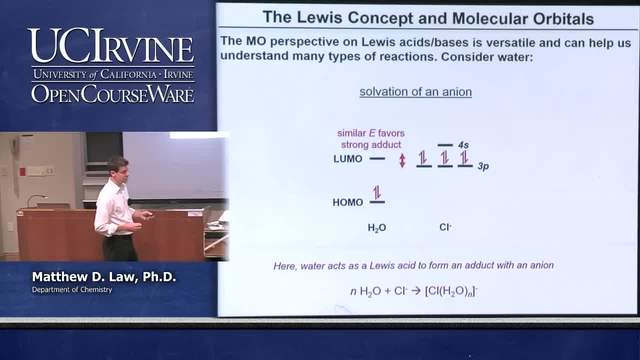 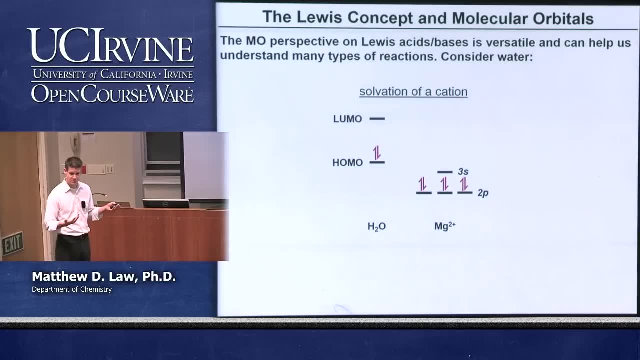 Right. The larger the anion, the more waters you're going to be able to fit around it. Okay, Now let's talk about water as acting in the opposite sense, As acting as a Lewis base instead of a Lewis acid, Right. 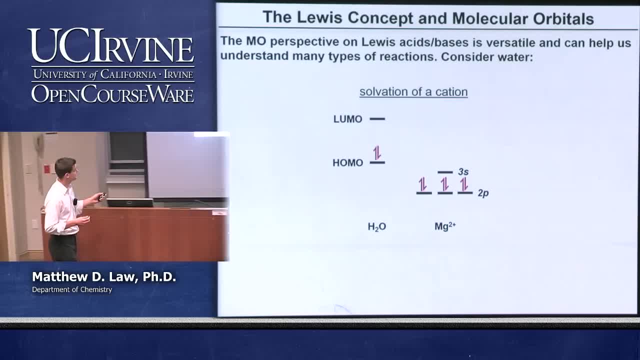 So it can be a base or it can be an acid, and it depends on what it's reacting with. Okay, So here's an example where water is in contact with magnesium: two plus Okay, Oxidized magnesium in the second oxidation state. 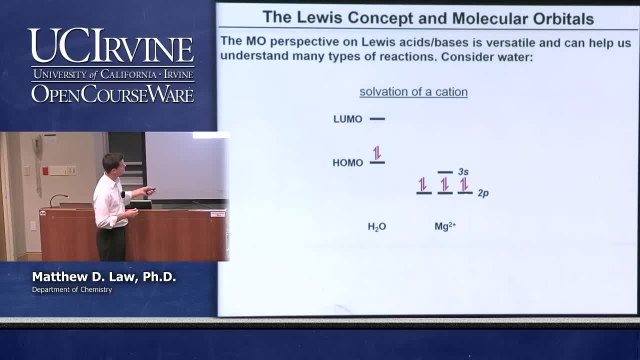 The homo of this is going to be two P's. The lumo just above the two P's is the three S. Okay, The water homo tends to be a little bit above the three S of magnesium, And so we can imagine water now acting as a Lewis base supplying these electrons in some sense to the magnesium. 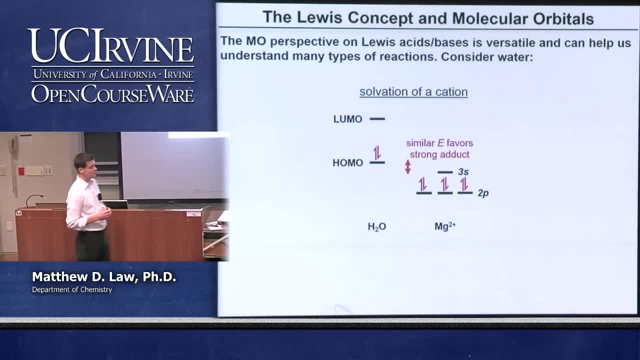 which will act as the Lewis acid. Okay, We have again a fairly small energy difference, So we're going to have adduct formation in general rather than redox reaction. Okay, And so this is the similar sort of reaction that we just showed. 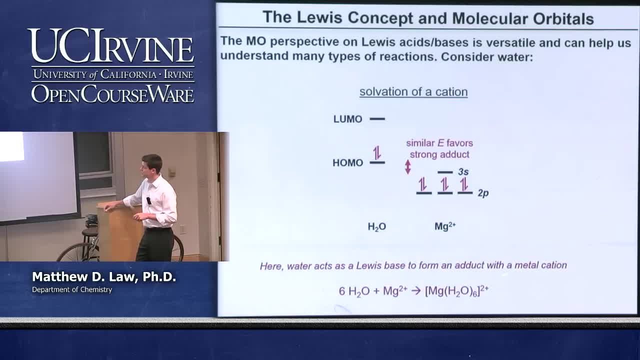 Water acts as a Lewis base. Okay, Forms an adduct with a metal cation, In this case forming six, a hexa aqua complex, where we have six waters around the magnesium ion. Okay, In this it's very similar to what we talked about with silver. 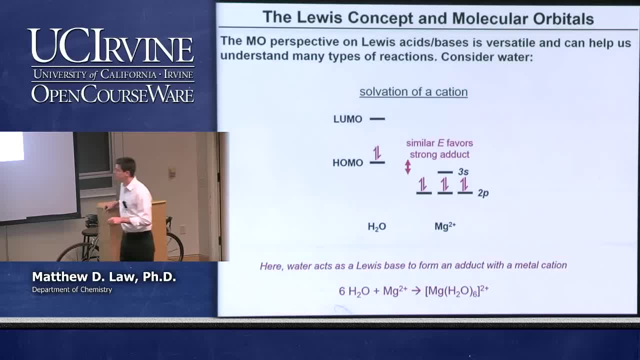 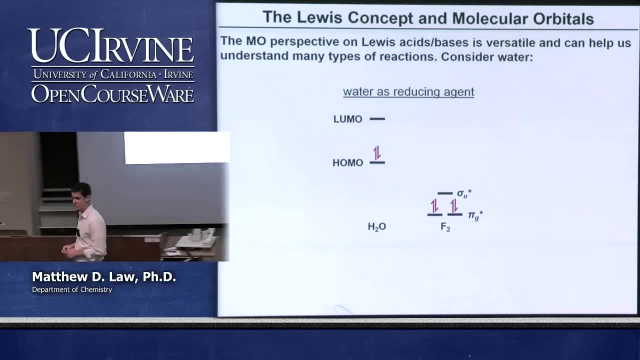 Right, We're forming a metal complex. The metal acts as a Lewis acid in general and water, in this case, is the Lewis base. Okay, Finally, the last possibility is if we have a very, very large energy offset in the reverse direction. 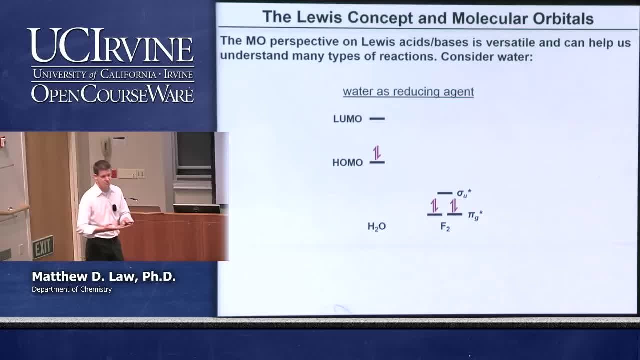 Now water can act as a Lewis base that's going to completely transfer electrons to the other reagent. In this case we're looking at F2.. Okay, So we bubble fluorine gas into water. What happens? Well, we know from the homonuclear diatomic MO diagrams what F2's frontier orbitals look like. 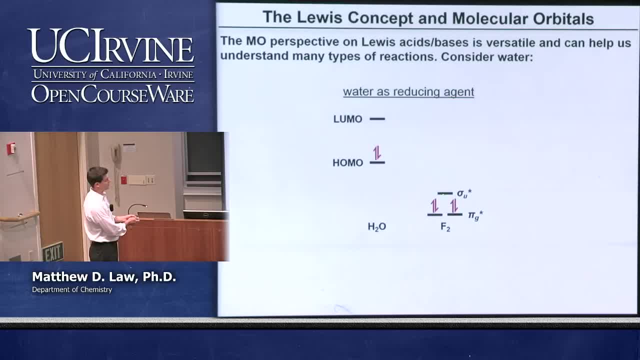 Okay, There's its HOMO, There's its LUMO, LUMO lying quite a lot lower than the HOMO of water, And so in this case we've got a large driving force for electrons to jump down to fluorine and form fluoride. 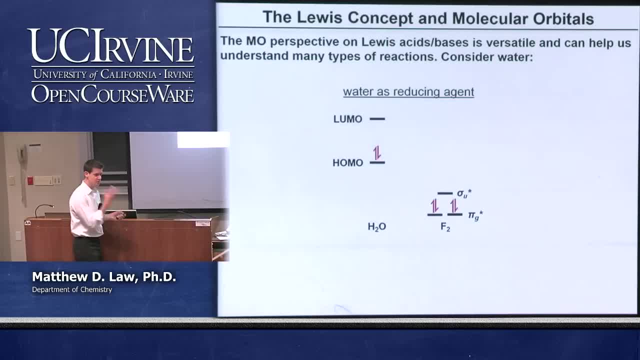 Okay. So again in your mind, you can think instantaneously: These electrons transfer, These electrons transfer to this anti-bonding orbital, making F2 2- for some ridiculously small period of time, if it happens at all- Okay. And then the F2 2-, just conceptually, is not stable and it breaks apart. 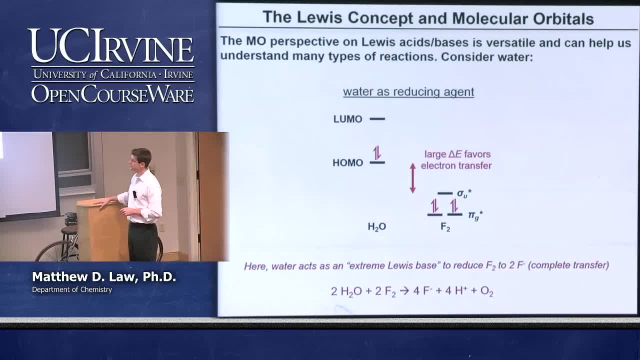 So what do you end up doing? You do a redox reaction here. where you take water, react it with fluorine, You reduce the fluorine to fluoride And you oxidize the oxygen in the water, in this case to O2.. Okay, 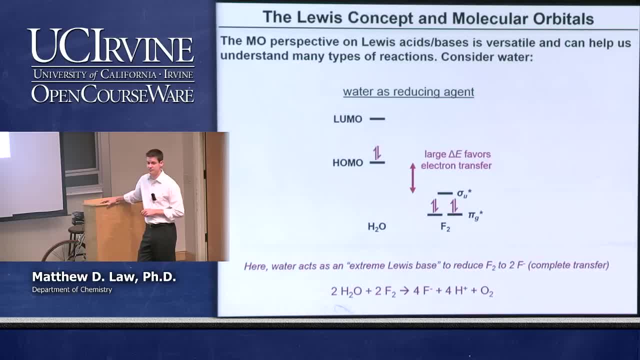 So neither the fluorine nor the H2O remain themselves after this redox reaction. Okay, And so if you have an idea about where the HOMOs and the LUMOs are for the two species that are interacting, you can get an idea about which one's going to act as the base, which one's going to act as the acid. 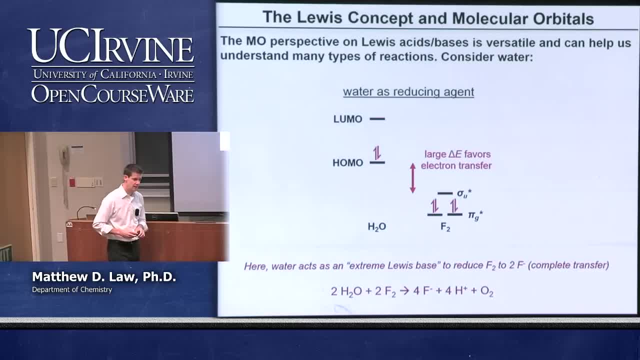 and what's going to happen in the reaction? Okay, Addict formation or complete electron transfer on the kind of outer edges of the possibilities? Okay, Questions about this. So the idea here is that many species are extremely versatile in their Lewis acid-base chemistry. 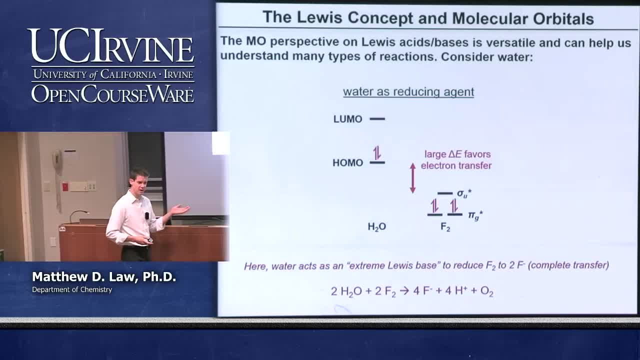 And even strong Lewis acids might meet a Lewis base that can overcome- or sorry, a Lewis acid that can overcome- their acidic properties and transfer them into a Lewis base. We'll talk about this a little later when we talk about super acids and super bases in Friday's lecture. 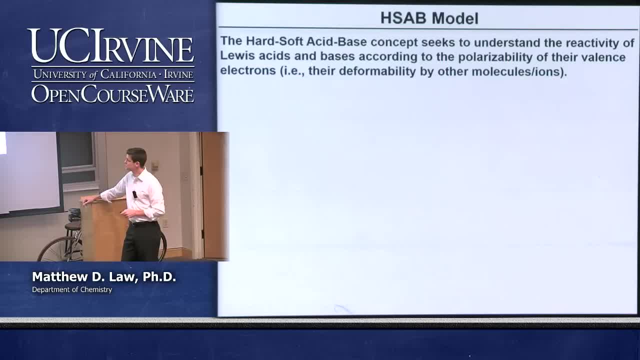 Okay, Okay. So if there are no questions, let's go forward. So there's an effort- there has been an effort since the 1960s to understand conceptually, kind of qualitatively again, acid-base reactivity, And one of the models, that is- we could call it semi-quantitative, is called the hard-soft acid-base model. 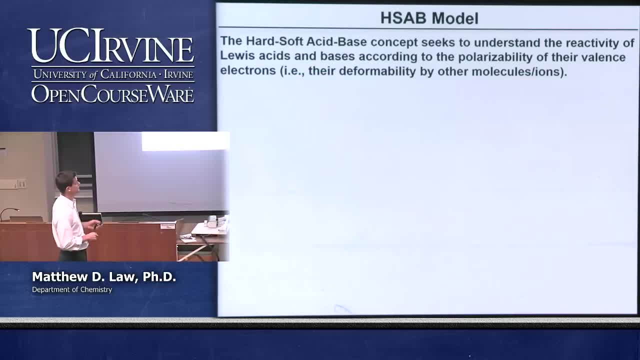 So this is the HSAB Hard-soft acid-base- Okay, Or the Pearson acid-base model, for the person that first developed the model. So this is an interesting concept, Hard-soft acid-base concept. We're trying to understand reactivity. 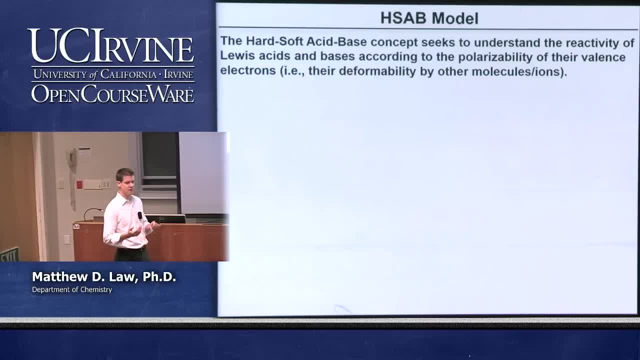 So, in general, we're trying to understand what the equilibrium constant is for a Lewis acid-base reaction, And we're going to understand this categorized species according to their polarizability, Okay, In other words, how much their valence electrons can move around. 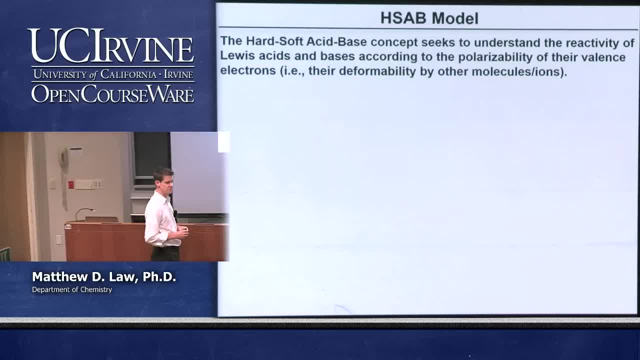 Move around in the molecule, How deformable they are, How floppy the individual species is. So if something is very polarizable, it's very deformable by an electric field. The electrons are movable and the molecule or the ion can be shaped and distorted. 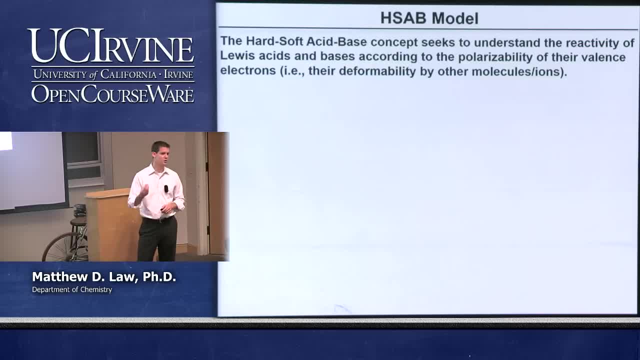 If something is not very polarizable, you can think of it as very hard. It's very immobile in an electric field in terms of its shape. It's not going to distort easily, It's not going to deform. So with this general idea of polarizability, it's possible to classify Lewis bases and acids according to whether they're hard and soft. 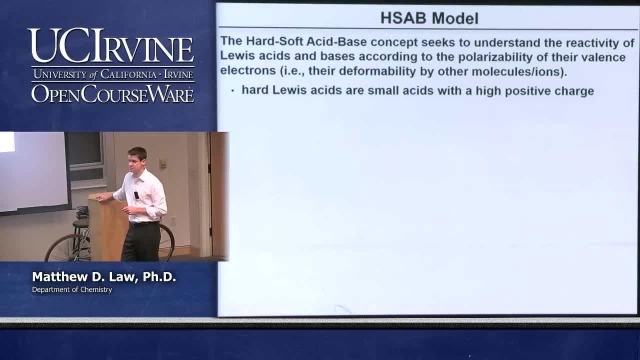 And the properties that we're looking for for a hard Lewis acid. things that are going to prevent it from being very polarizable are as if it's very small and if it has a large charge on it- Large positive charge usually Okay. 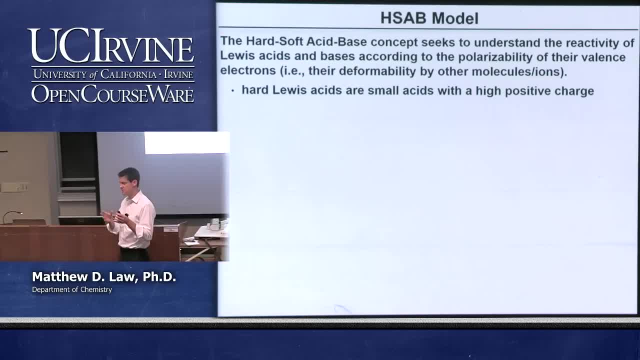 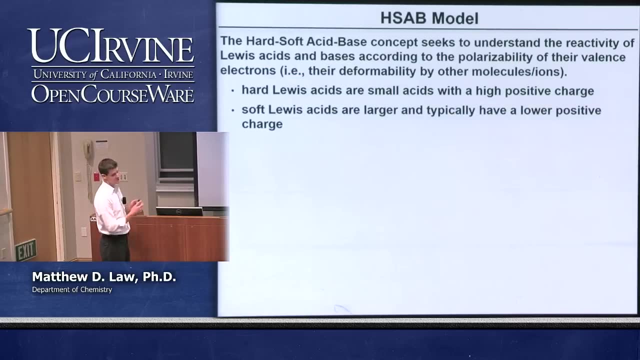 That makes the ion cloud, the electron- sorry, The electron cloud, the electron density around the object difficult to perturb If it's small and if the electrons are experiencing a strong positive charge. So that would be a hard Lewis acid. A soft Lewis acid is the opposite. 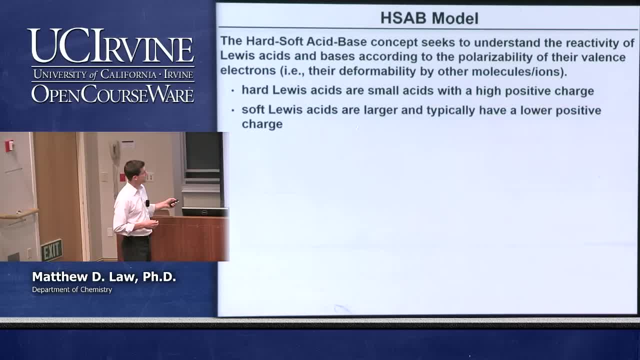 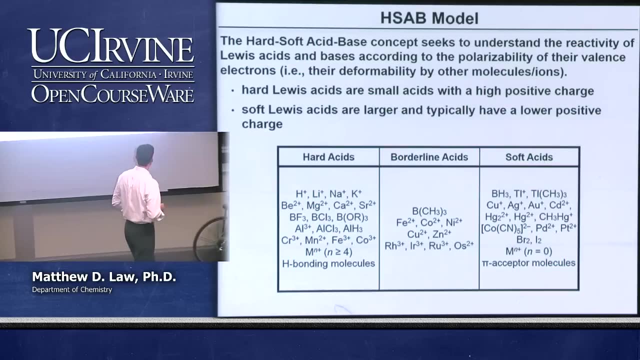 It's big, It's floppy, So it's big. It typically has a low positive charge or no charge on it, And so the electrons can be more distorted. The electron cloud is more distorted by an applied field. Okay, So we can tabulate, classify lots of different basic Lewis acids according to whether they're hard or soft. 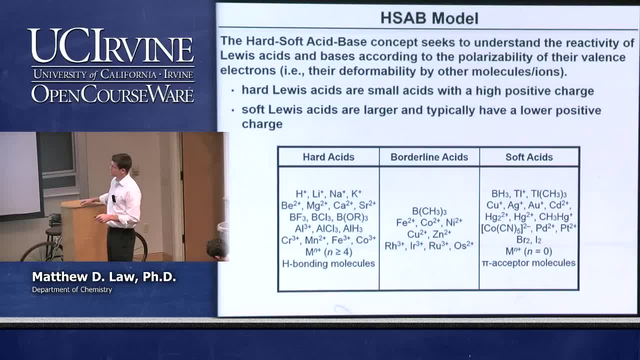 Or whether they're sort of in the middle. So hard acids are those that are small and have a high positive charge. So small includes things like protons, lithium, sodium, potassium, Those things that have a large positive charge- chromium-3, iron-3,, cobalt. 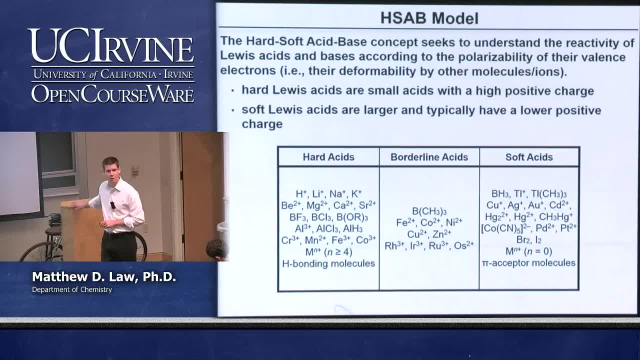 Metal ions that have charges of four or more. Those are going to be hard Lewis acids. And then there are other things. BF3 is considered to be a hard Lewis acid because it's fairly small. It's got these electronegative atoms associated with it. 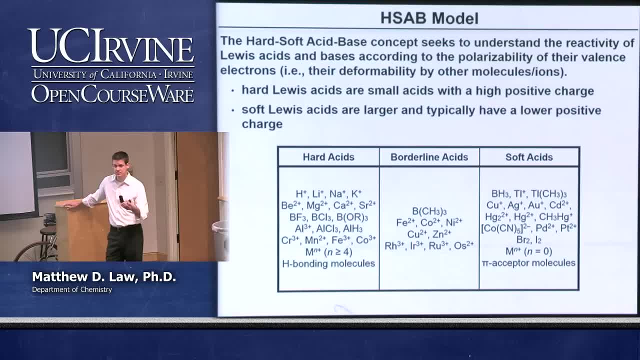 On the other side of the table we have the softs. These are big low charge floppy. So you have things like low charges, copper, single charge, silver, gold. Mercury is always a soft acid, Whether it's by itself or whether it's methylmercury or something else. 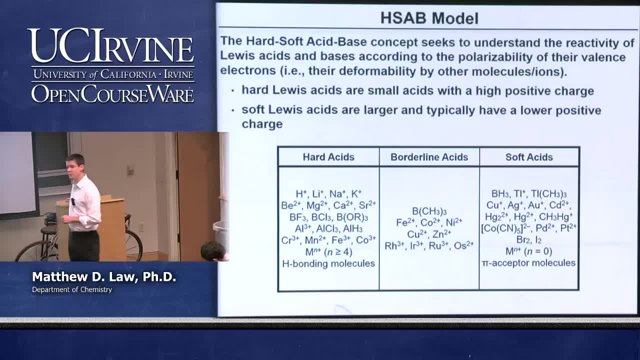 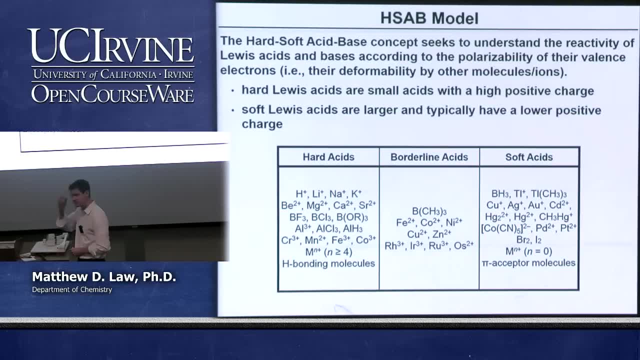 You have things like bromine and iodine- Molecular bromine and iodine are considered to be soft Lewis acids- And there are a variety of others too. And then we have intermediates, And probably the only intermediate that we're going to come into contact with really is zinc-2.. 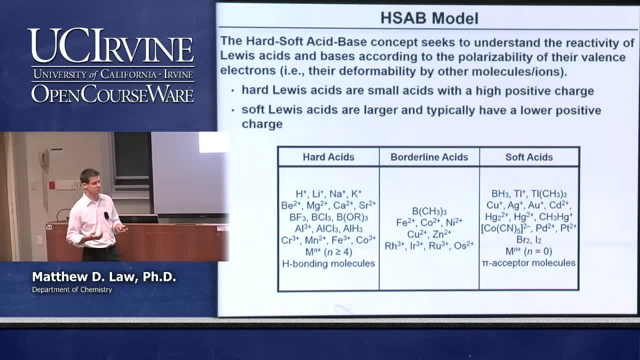 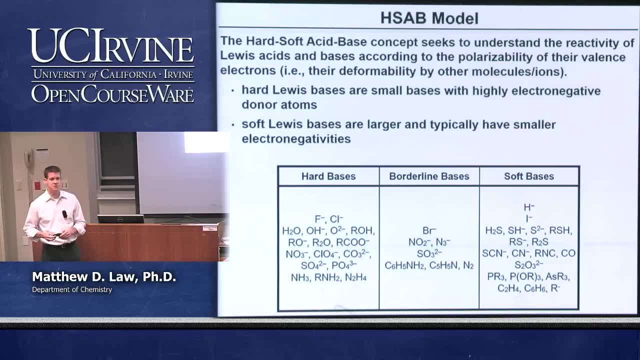 But these are sort of of course in the intermediate size regime and intermediate charge regime. So we have hard and soft Lewis acids. We also have hard and soft Lewis bases, And the idea is exactly the same: Hard Lewis bases, small, with a highly electronegative element. 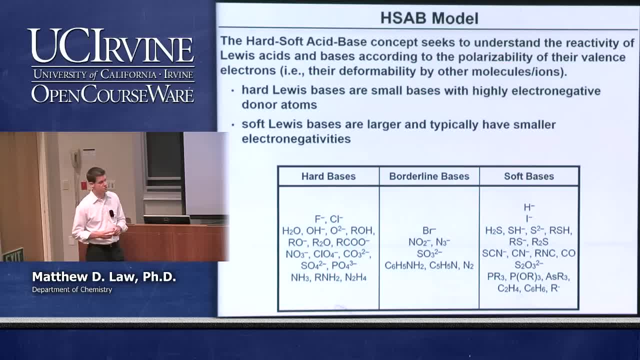 Soft Lewis bases are large, typically have a smaller charge on them and smaller electronegativities. So the most important of the hard bases are those that are very tight, very compact Fluoride Chloride. These are very hard bases. 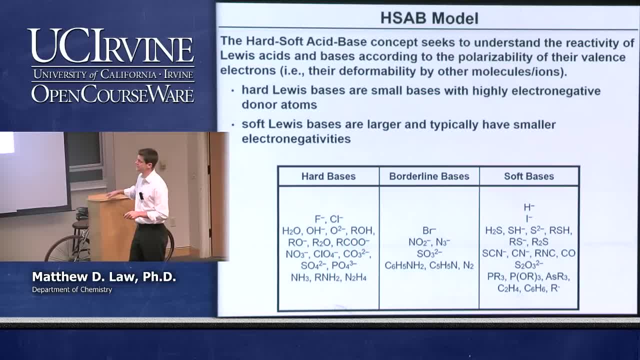 But there are others. A hard base is water, And that's an important hard base, And it's deprotonated species. OH- and O2- are hard, And then quite a lot of organic molecules, Alcohols, carboxylic acids, carboxylates. 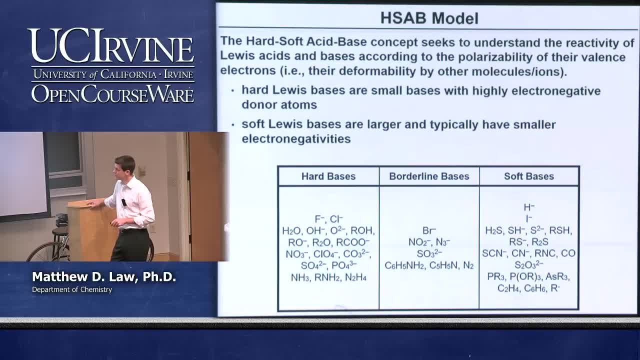 Things like sulfate, phosphate, And then we've been talking about amine, ammonia here. That's also a hard base. The soft bases are those that have you know, larger size right And less electronegativity. So hydride iodide is a nice soft Lewis base. 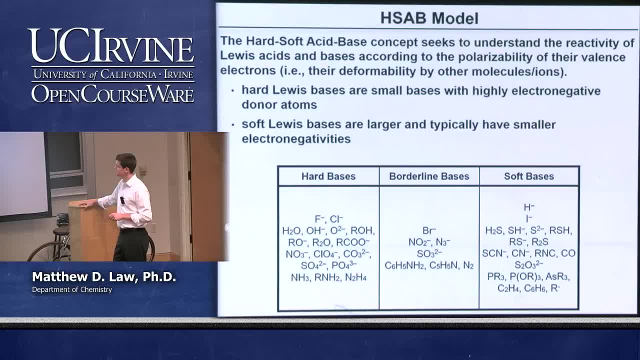 And then there's a bunch of others, Some that we'll come across, but many that we won't. So some molecules, like benzene included, are soft bases. We're going to see an example with benzene later today, And then again, of course, we have the end members, the hard and the soft, but we have intermediates too. 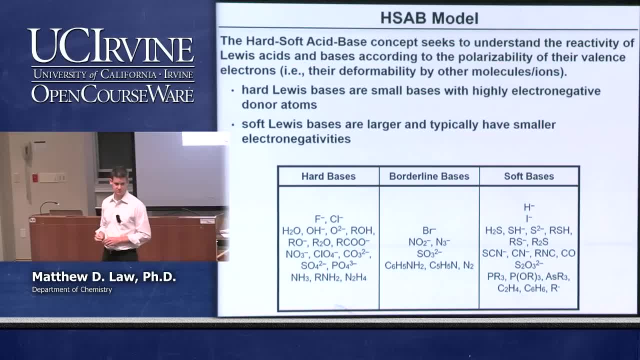 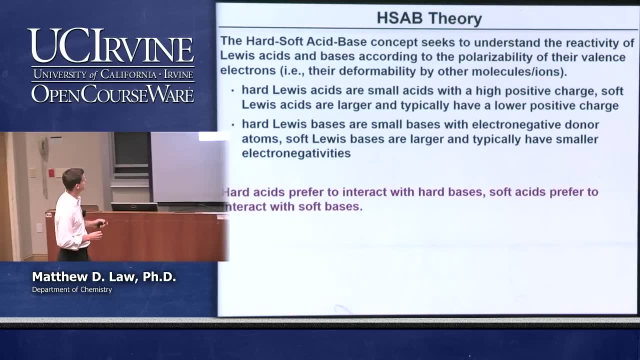 And these are just qualitative categorizations. So we can assign actual semi-quantitative values to these, And I'll show how we do that in a little bit. Okay, So what? So we can have hard and soft acids and bases. What's the idea? 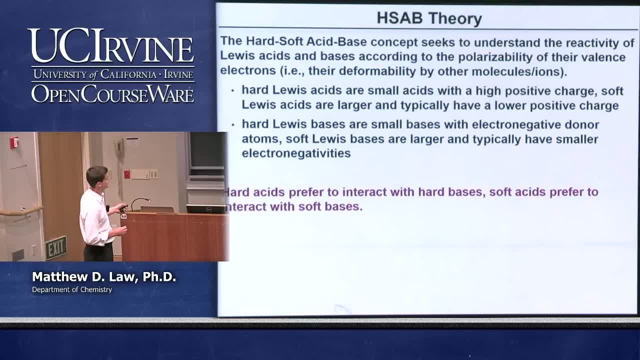 This is just a regurgitation of what hard and soft acid bases are. The idea here is that- and this is what Pearson struggled for a long time to convince everyone of- And it's basically been accepted as a very useful tool In inorganic chemistry. 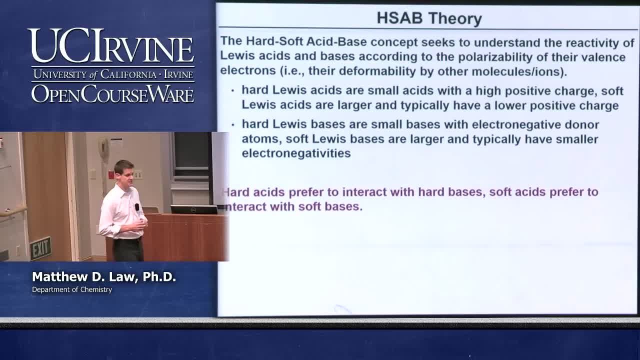 Hard acids prefer to interact with hard bases And soft acids prefer to interact with soft bases. That's the general idea: Hard likes hard and soft likes soft, And so you will expect large equilibrium constants and strong ad formation when you have hard-hard and soft-soft. 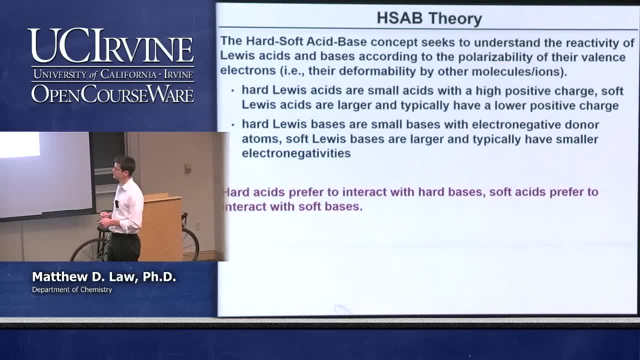 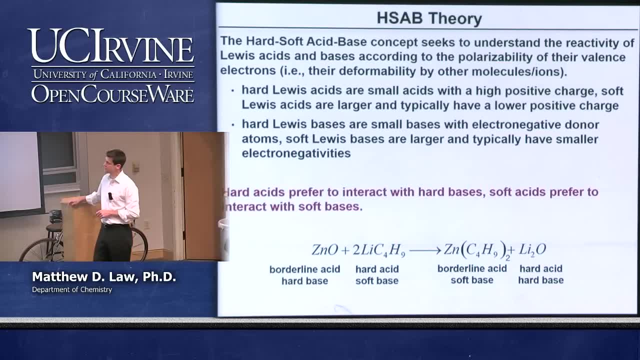 Otherwise, if you have mixtures between hard and soft, we expect poor reactivity and smaller equilibrium constants for those reactions. So here's a reaction that we can digest in terms of hard-soft, acid-base chemistry. So this is a reaction of zinc oxide and lithium, n-butyl lithium- here. 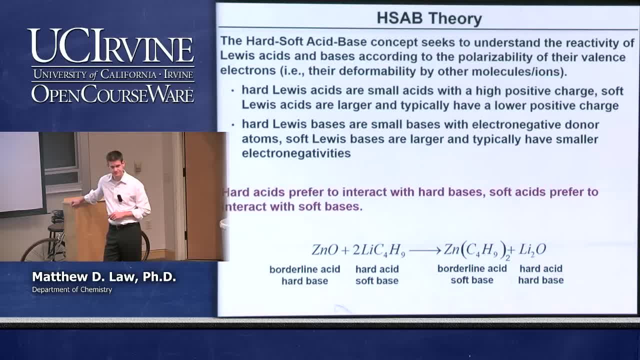 Going to zinc and n-butyl lithium, zinc and lithium oxide. So probably you've seen lithium chemistry and organic chemistry right, Also some related chemistry in the group twos, So we can look at each of these individual species and categorize them. 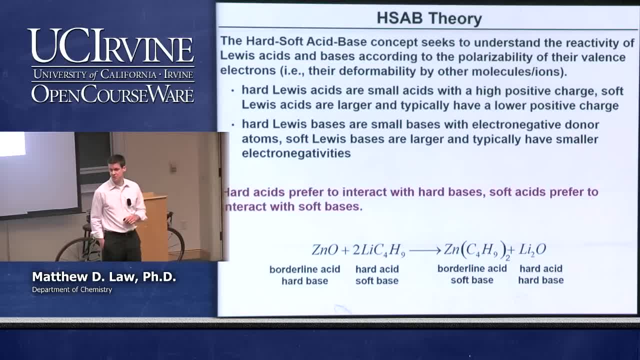 We can categorize them as a product between hard or soft-loose acid-base Zinc oxide. we have a borderline acid, which is zinc two plus, with a hard base which is O two minus. We can look at the n-butyl lithium here. 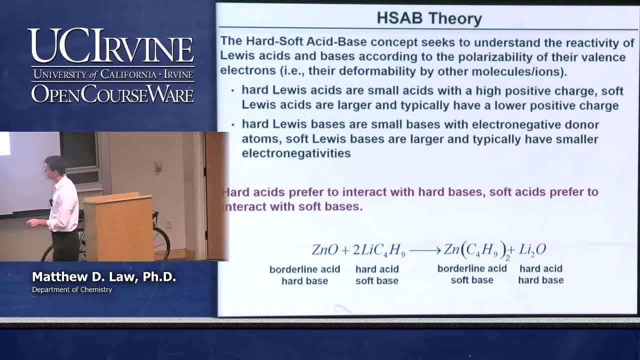 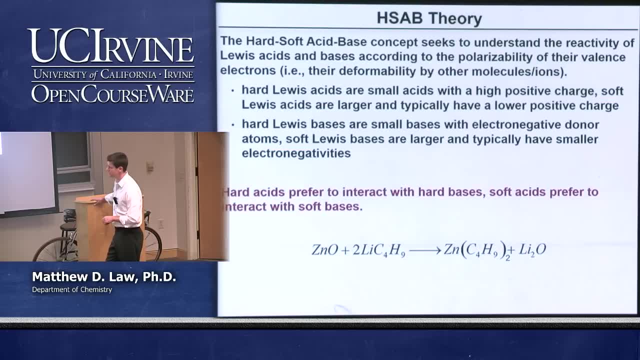 Lithium is a hard acid. It's a small cation, N-butyl lithium- soft base. This is not something that I highlighted, but if you go back to the tables, I won't do that. But if you go back to the tables, you'll find that the alkyls are going to be soft. 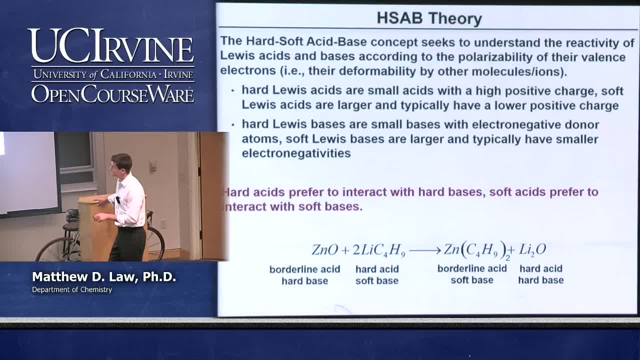 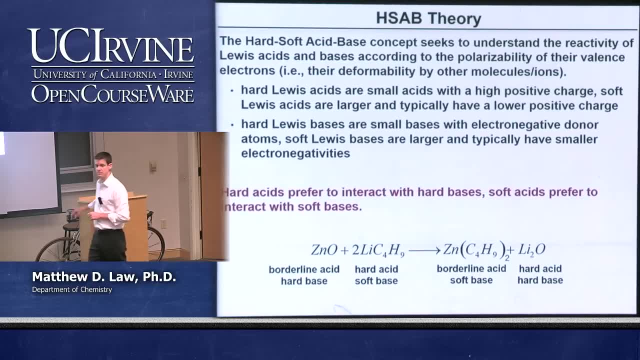 Classified as soft Forming, in this case a borderline acid with a soft base right Where we just exchange And a hard acid and a hard base. And this is the critical thing here. We have hard and soft mixtures here and in the products we have one in particular, that's a hard acid with a hard base. 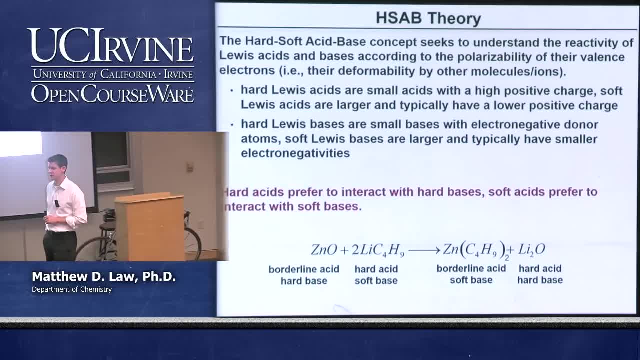 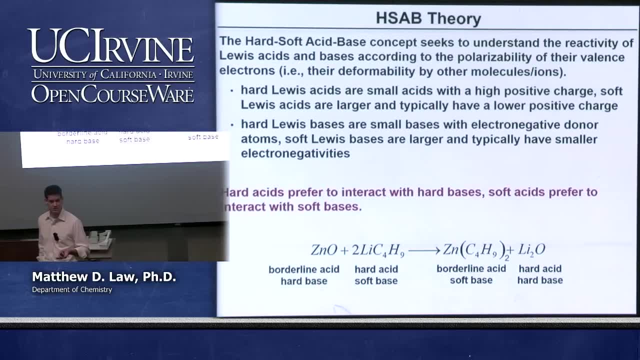 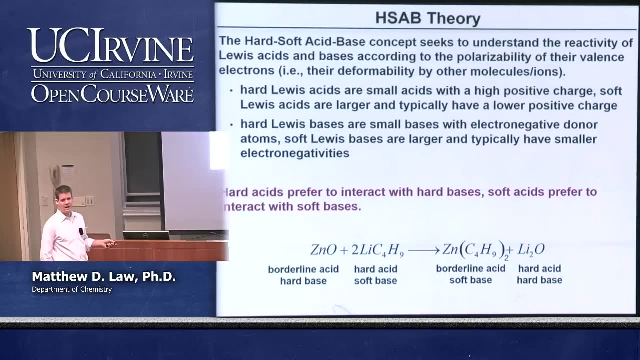 That's a very favorable interaction in the hard-soft-acid-base picture And this is one of the driving forces, if not the main driving force- for this reaction going to near completion In the hard-soft-acid-base model. We'll explain in a little bit why there would be such a driving force. 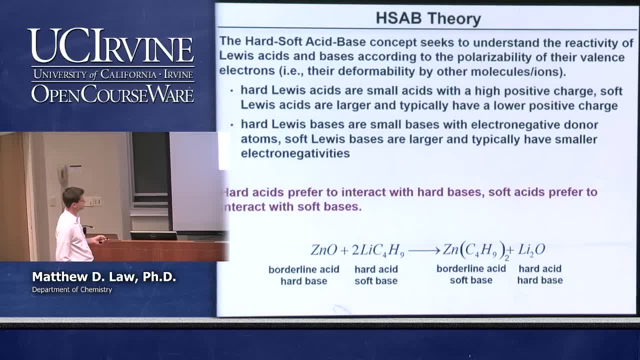 Why hard-hard and soft-soft are preferred. But this is the general idea. We can decompose each of the reagents into whether they're hard or soft, acid or base or a complex of the two, And then determine what kind of reactivity to expect. 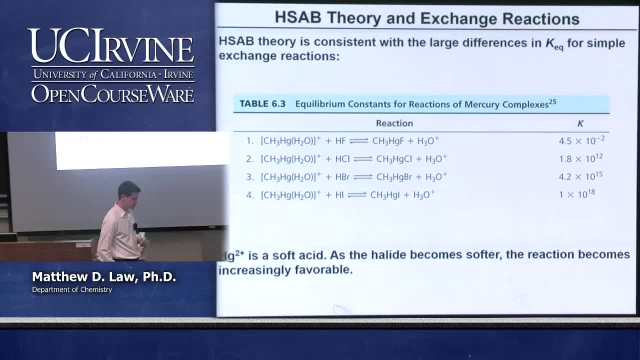 So the hard-soft-acid-base picture is pretty good at describing trends in reactivity And there are several of these trends in your book that are described. One of them is looking at the equilibrium constants for exchange reactions. In particular, we have exchanges like this: 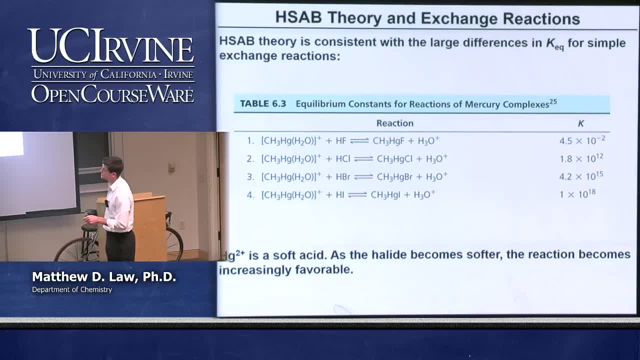 So what we have here is methylmercury that's got a water associated with it, And we're reacting methylmercury with one of the acids HF, HCl, HBr or HI, The halide acids. Methylmercury is a soft base. 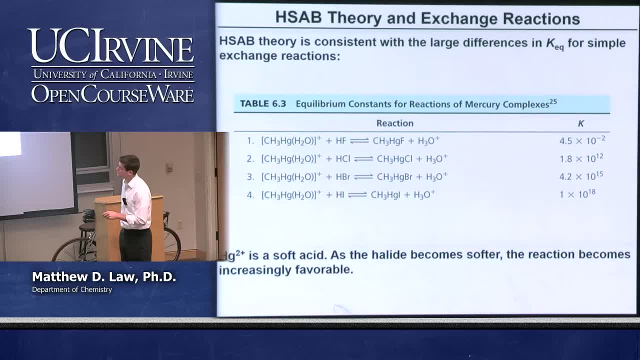 Soft acid I mean. And so what we're doing here is we're changing the base from fluoride to chloride, to bromide to iodide, Going from hard to softer to softer to softer, as we get larger and larger ion size And as we make that element less and less electronegative. 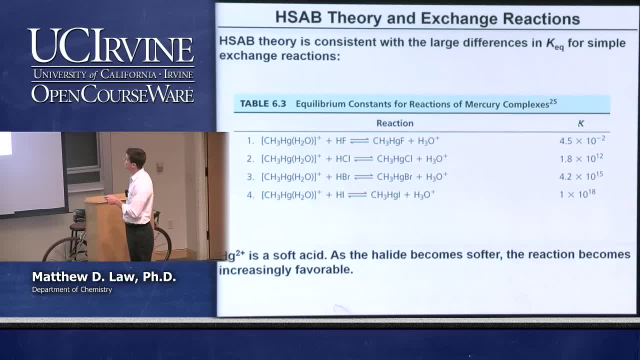 And what we see when we do that. when we go from HF to HI, the equilibrium constant goes from very small to very, very large, And so we can understand this kind of trend in terms of HSAB, As the halide becomes softer, because mercury 2 plus is a soft acid. 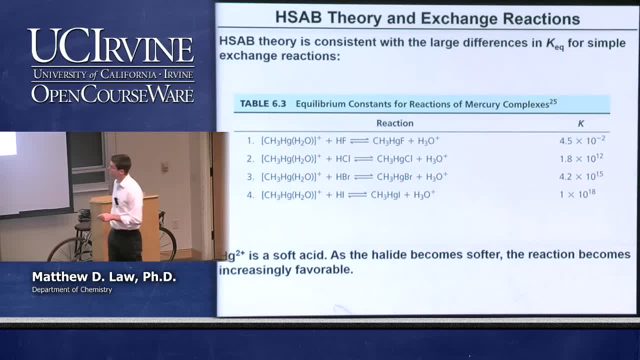 As the halide becomes softer, the reaction becomes increasingly favorable, Because we have here a soft and a hard, And then we have soft and softer as we go down. Finally, in four, we have the softest and softest situation And that leads to the largest equilibrium constant. 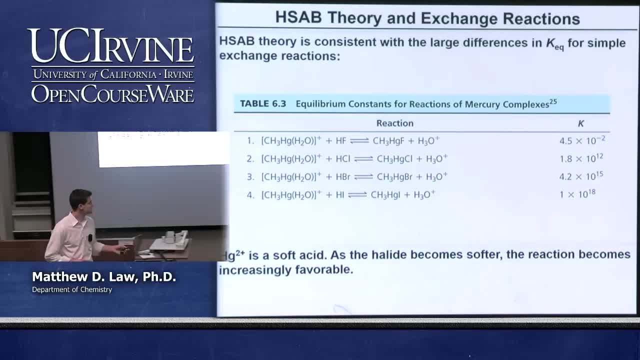 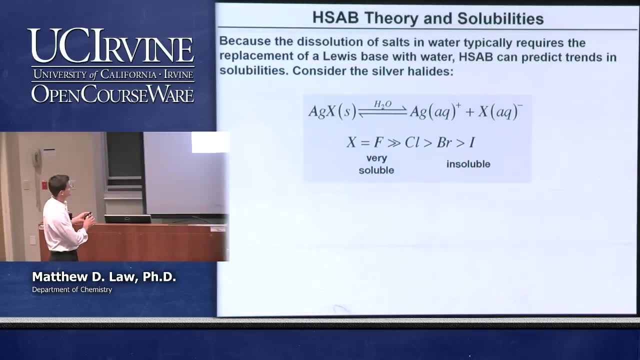 So that's one way to understand this kind of reactivity. We can look again at another trend. Let's look at the dissolution of silver halides in water, Forming silver plus and halide. And we can look at the solubility trends when X goes from fluoride all the way to iodide. 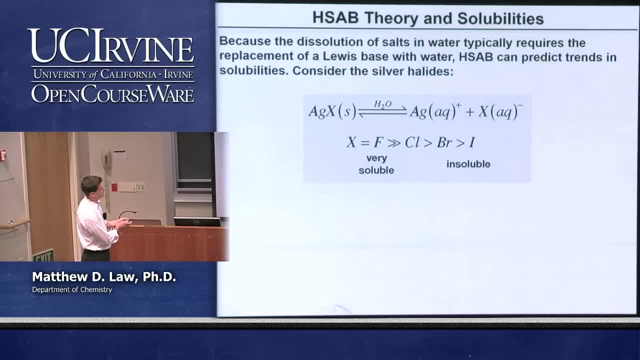 With fluoride we have a very soluble situation And we go progressively more insoluble as we go down the periodic table. Why would this be? Well, we can first classify the kinds of bases that we have here. Fluoride and chloride are hard bases. 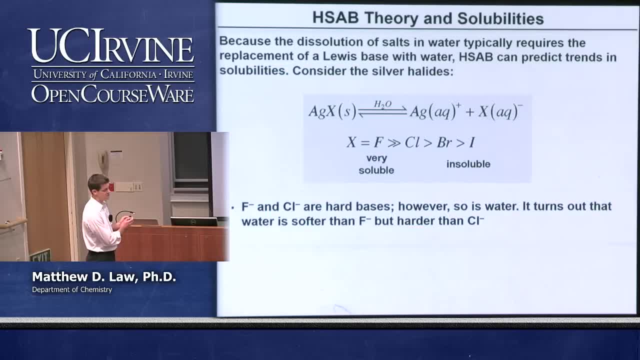 Water is also a hard base which we need to keep into consideration here, Because we've got the dissolution, basically as a competition for the silver between water and the halide. So fluoride, chloride and water are hard bases. It turns out that water is a little bit softer than fluoride. 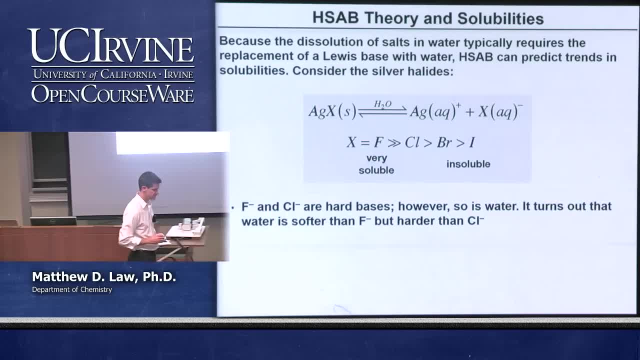 So water sits in between fluoride and chloride. in terms of hardness, We know that bromide and iodide are soft because they're big and floppy. And so the question is, what about silver plus? Well, we know silver plus is a soft acid. 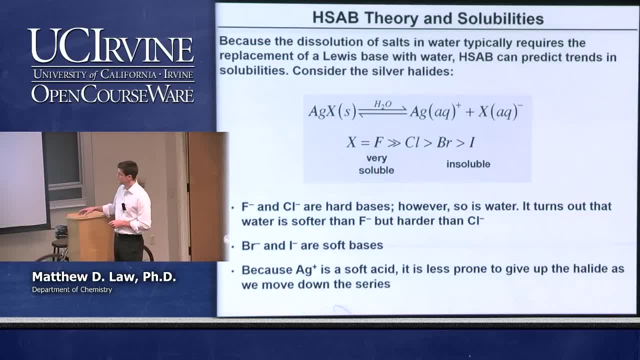 Small charge, fairly large ion. So it's going to be less prone to give up the halide as we move down the series. In other words, as we go from here to here, it's going to be less and less soluble Because we've got a soft situation mixed with a hard. that's going to be a very weak interaction. 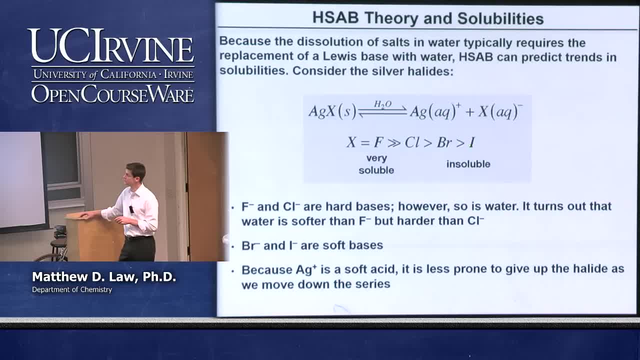 So it'll dissolve pretty easily. But as we come more down the periodic table we go from soft-hard to soft-soft in this direction. The interaction between the silver and the halide increases in strength And so we get less solubility of those species. 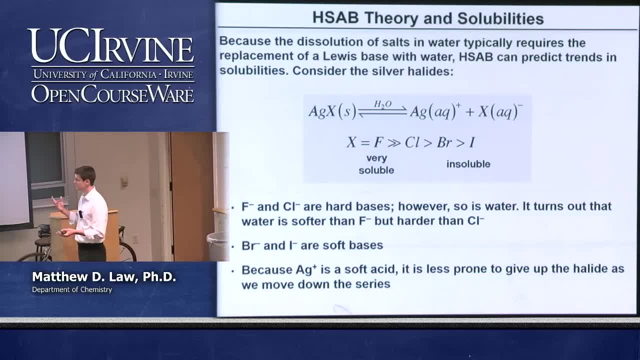 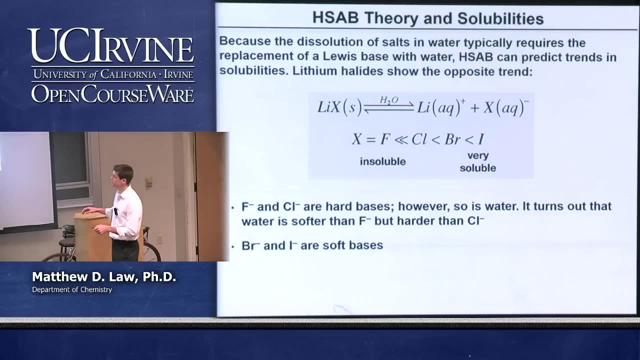 So it's again having a soft acid mixing, with softer and softer bases being more preferred. Same sort of idea. but what if we switch the cation? What if we have lithium halides instead of silver halides? Now we expect the opposite trend, because lithium now is a hard acid. 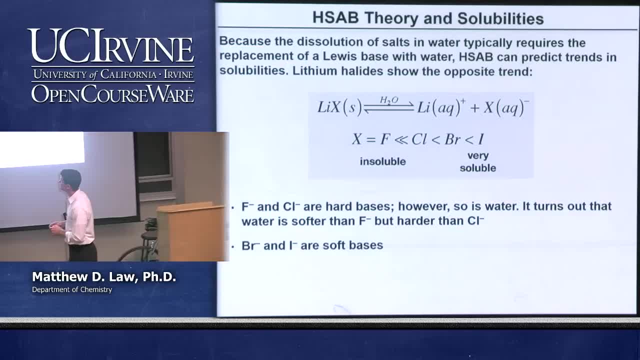 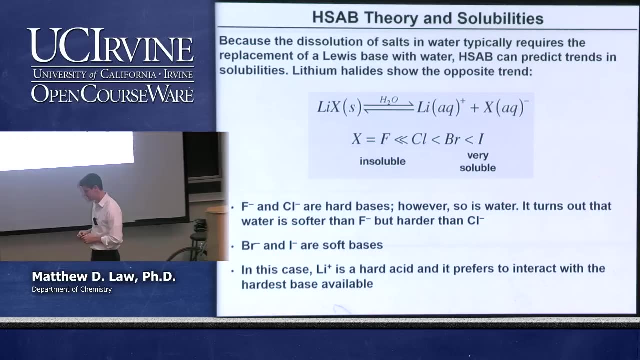 Small little lithium hard acid, And so what we should have now is the most insoluble species being the hardest base And the least or the most soluble species here being the softest base. So it just is the opposite trend of what we just described for the silver halides. 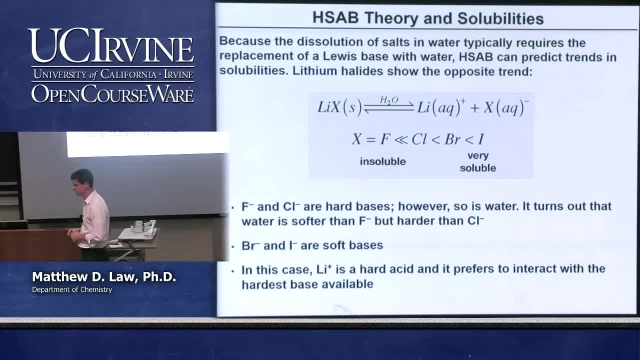 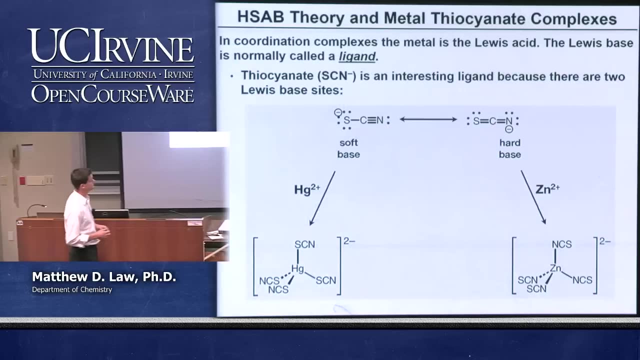 So lithium, being hard, prefers to interact with hard, And so the solubility of the lithium fluoride is going to be very low. So that's another example of where this kind of idea, this concept, can be helpful. Let's look at another one. 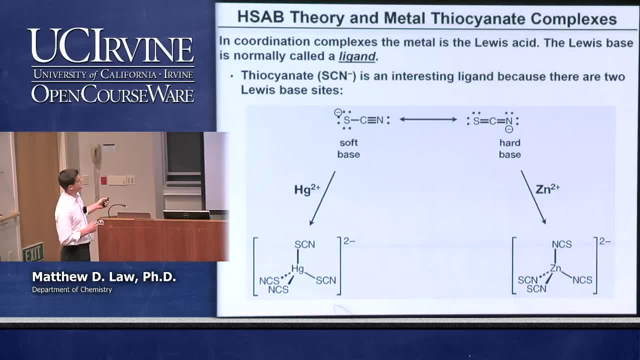 We can look at how ligands bind to metals in terms of hard-soft acid-base concepts, And this is a very common way to think about what sort of products you're going to generate in organometallic chemistry and inorganic chemistry. Looking at metal complexes, 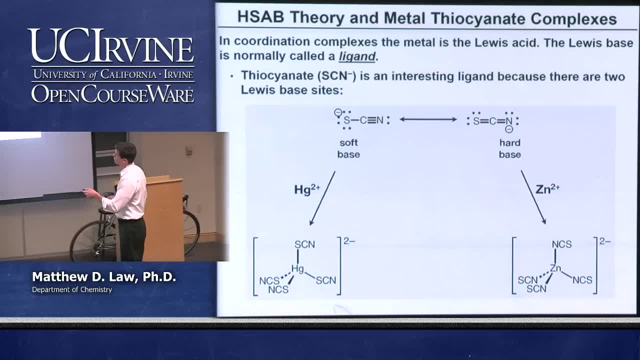 So just to remind you coordination complexes, we have a metal, one or more, That's the Lewis acid. Lewis base that comes in Donating electron pair is usually called a ligand. Thiocyanate is one such ligand. that's very interesting because it can either bond through the sulfur or through the nitrogen. 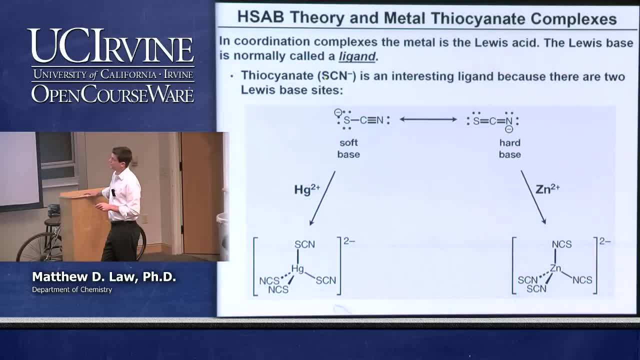 And so when would we expect thiocyanate complex to bond through sulfur versus nitrogen? Well, it turns out that the sulfur is much softer than the nitrogen side, because the sulfur is quite a bit larger, And so if the sulfur comes in to bind, that's considered a soft base. 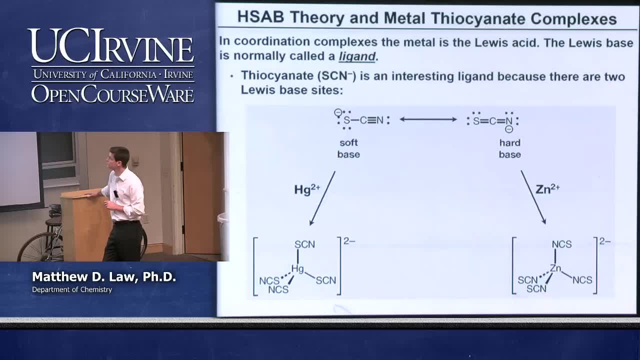 Whereas if the nitrogen comes in head first, that's going to be a hard base, And so you expect to have metal complexes in which the sulfur is directly connected to the metal, when the metal is also soft, when the metal is a soft acid. 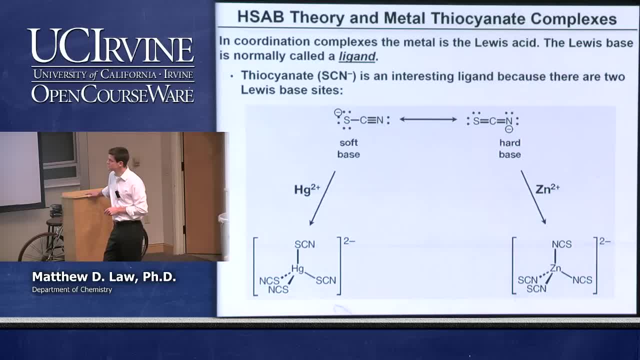 So mercury is a great example of that Very, very large, soft ion And in mercury complexes we're typically going to have the thiocyanate binding with the sulfur rather than the nitrogen Rationalized, again because of this soft, soft preference. 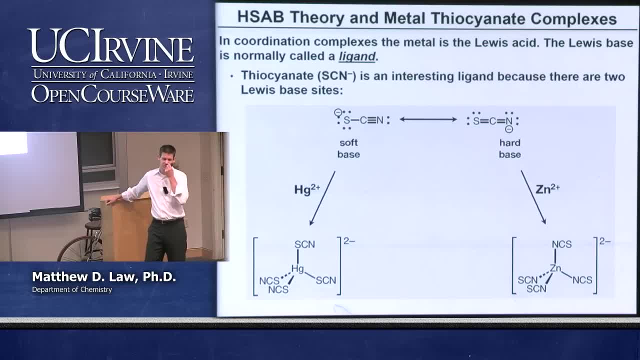 If we have instead zinc complexes, zinc being kind of borderline, but in this case we're going to call it hard, more hard than soft. The zinc complexes have the binding through the nitrogen, because we've got a hard, hard preference in this case. 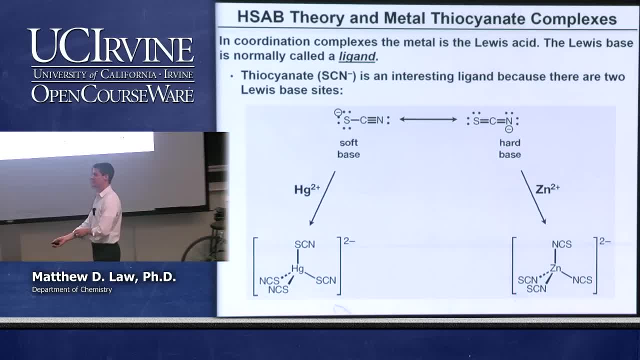 Does this always work? Of course not, But it works fairly frequently And it suggests that there's something to this idea. There's some physics, some physical reality that's behind this concept. that is tangible, that's real. It may be interpreted in a weird way that seems very wishy-washy. 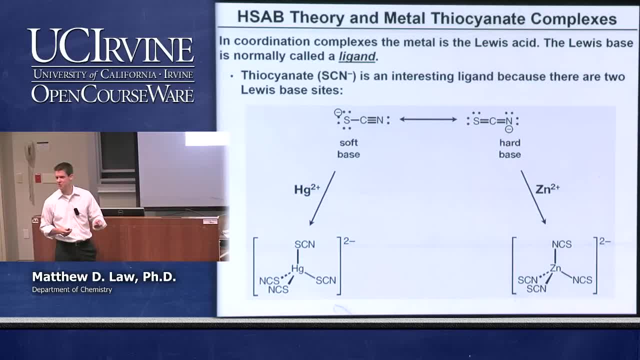 But Pearson is on to something here. Okay, Okay, And this again, this kind of idea. Okay, This idea is used very frequently in understanding metal complex formation. You'll talk about this later, when you talk about isomers of metal complexes. 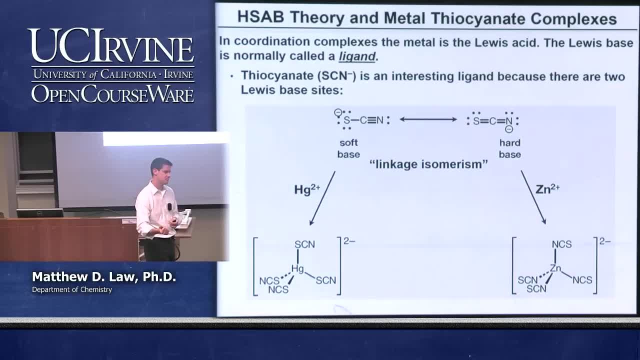 But this is called linkage isomerism, where it can come in with one foot or the other, Or one hand or the other, The sulfur or the nitrogen, Questions about these examples? This is just to convince you that you know there is some reality to this idea. 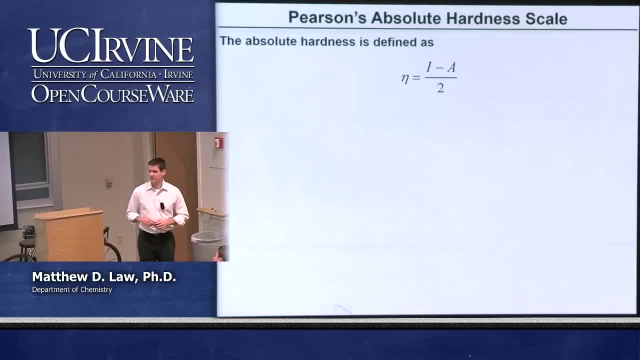 Okay, Let's quantify it a little bit. Okay, It can be quantified. We would call this semi-quantitative because it's a model. It's not generated from first principles, from basic physical principles. We can quantify and Pearson quantified the absolute hardness in the following way: 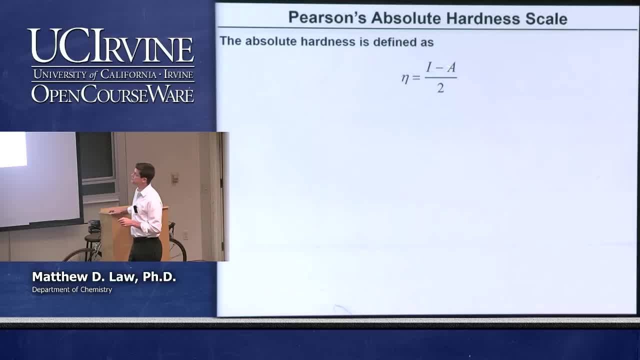 The absolute hardness. eta is just half the difference of the ionization energy and the electron affinity. Okay, So you take the ionization energy, subtract the electron affinity, divide by two And that's your absolute hardness. Why do we do this? 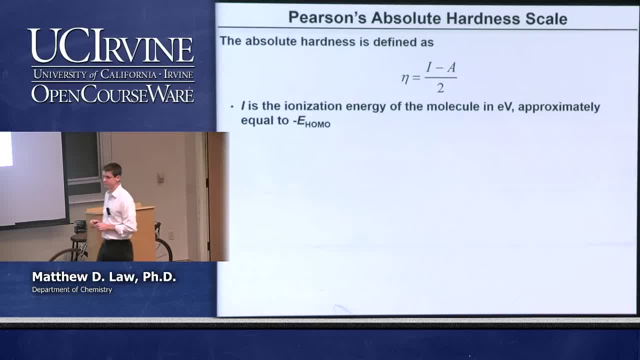 The ionization energy I is basically equal to the negative of the HOMO energy. So to remove an electron we have to remove it from the highest occupied molecular orbital, That's the lowest ionization energy. So the ionization energy is approximately equal to the negative of the HOMO. 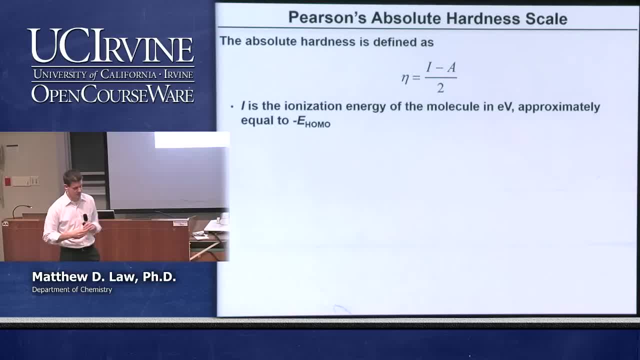 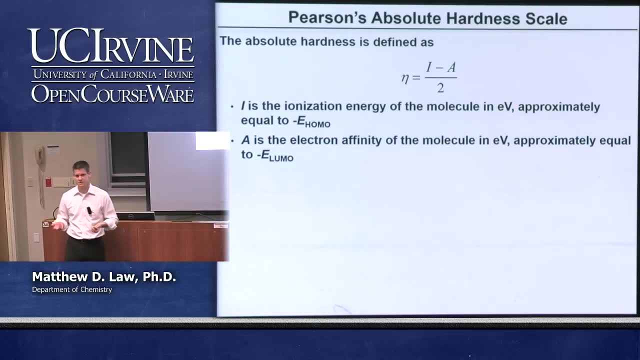 Remember that the HOMO values are all negative because we've got zero as kind of the reference level. So that's the HOMO position. Of course, the electron affinity is the LUMO position. All right, So that electron that's grabbed by the molecule or species is going to sit in the lowest unoccupied molecular orbital. 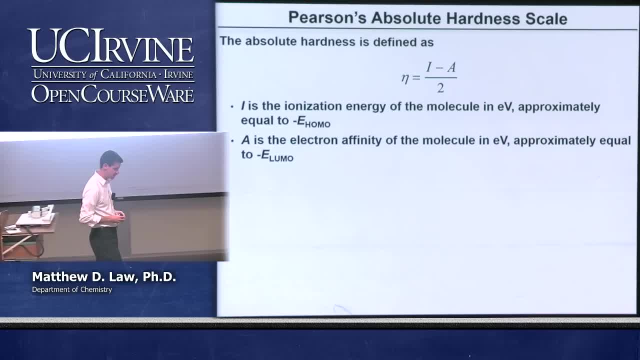 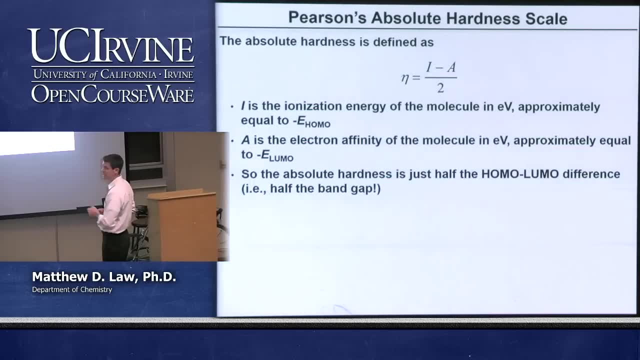 So we get a pretty decent estimate of what the LUMO is going to be, And so what this is telling us is that we have the hardness corresponding to half the HOMO-LUMO gap, half the HOMO-LUMO distance, half of the band gap, if you want to call it that. 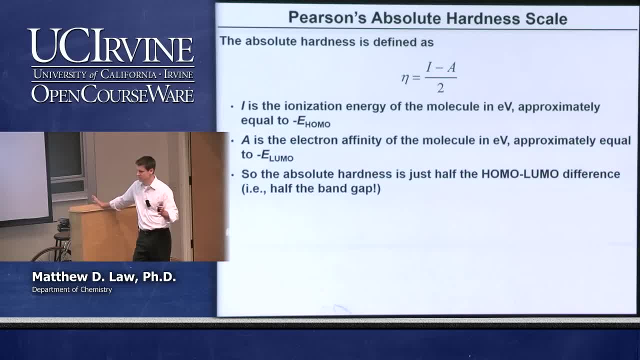 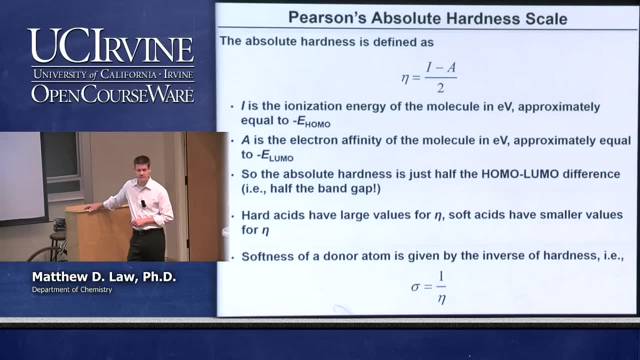 Of course that doesn't make any sense with molecules, but I always think in terms of the band gap. Okay, Of course, hard acids have large values for eta, Soft acids have smaller values for eta, And if you want to talk about softness instead of hardness, it's just the reciprocal, just the inverse. 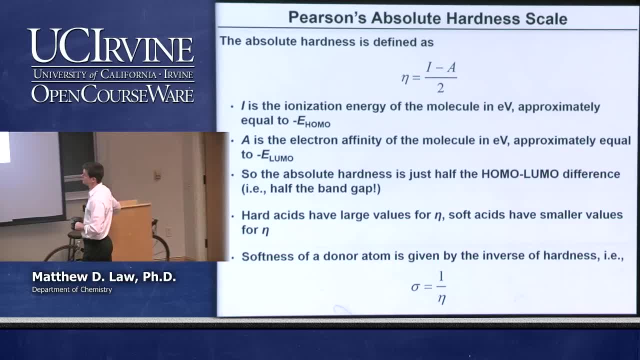 So what, of course, is hard is not soft. Okay, All right, So you can tabulate. The nice thing about this is that you can actually measure the ionization energy, the electron affinity. You can calculate it, and so forth. 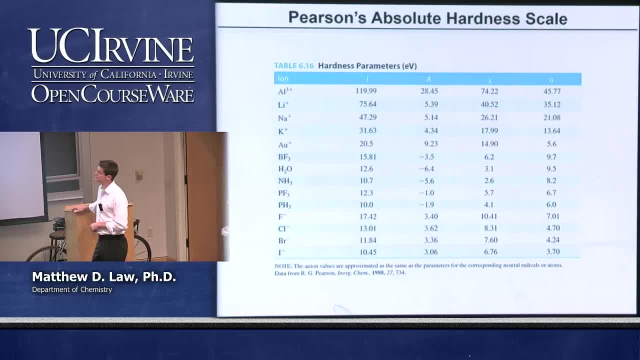 And so you can make tables then of the hardness parameter, And this is a table from your book, Okay, And so you see here some that have: here's the hardness parameter. here, Here's ionization, energy, electron affinity: Here's the hardness. Some ions that are very hard include those that we would expect: Aluminum 3 plus a very small ion, huge positive charge. This is going to be a very hard cation, a very hard acid. We've got some that are still hard right: lithium, sodium, potassium. 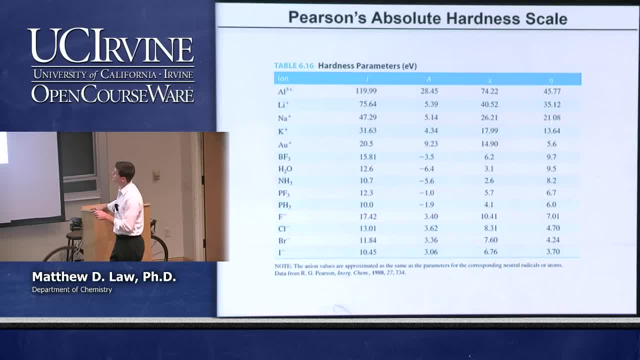 We said all of those are hard. These are pretty big values for eta. Okay, So as we go down, let's say gold, that's a soft acid, And look at the size of the eta: Okay, 5.6.. 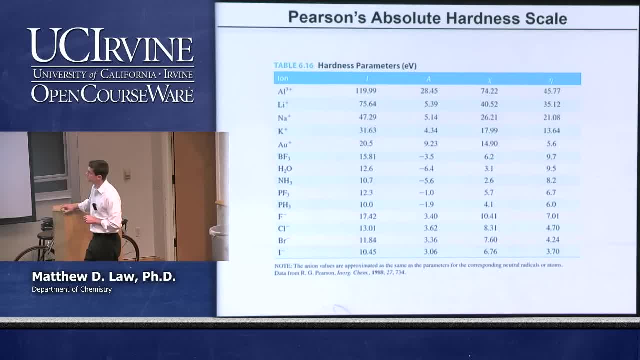 Okay, So much smaller than some of the harder ions that we've compared it to. We can look at some of the bases too. So here's fluoride, chloride, bromide iodide, And you can see that you go from 7 down to 3.5 or so. 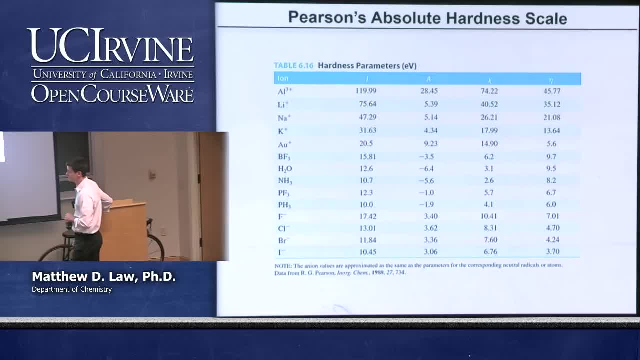 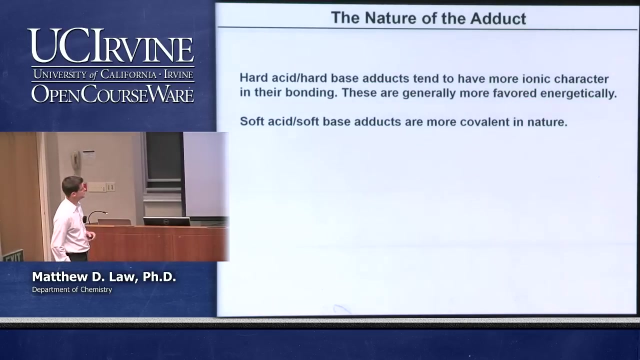 Okay, As we go down the periodic table here. So this has a relationship to the atomic energy levels or the molecular orbital energy levels, Which is nice because those are measurable and they actually have chemical significance. Okay, So let me just close in the last minute or so by briefly describing why hard-hard is preferred and soft-soft is preferred. 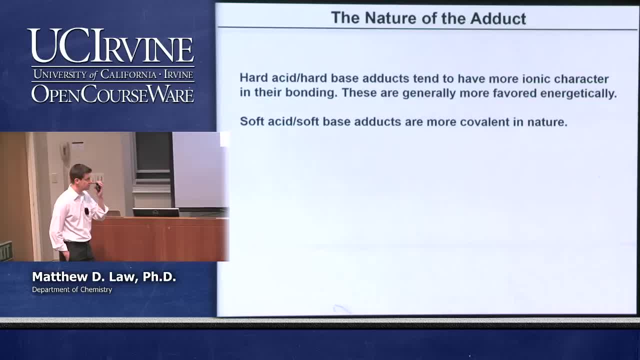 We'll get into this in a little bit more detail on Friday because I don't have time to describe it in totality right now. But the idea is that hard-hard interactions are basically ionic interactions. Okay, You have an ion that's coming in, that's not perturbable. 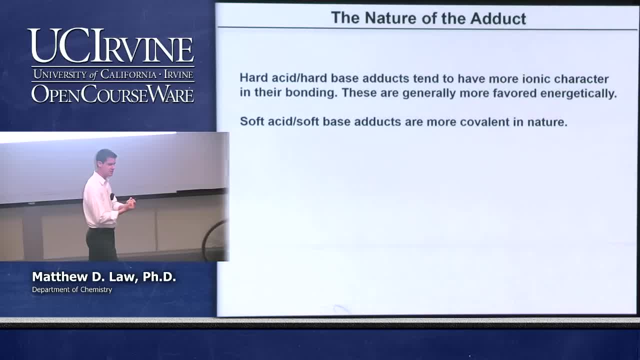 You have another one that's coming in, that's not perturbable. You're not going to share electron density, You're going to have ionic kind of bonding. Okay. So you have good ionic bonding when both are hard. The flip side: if you have soft-soft, those are highly polarizable interactions. 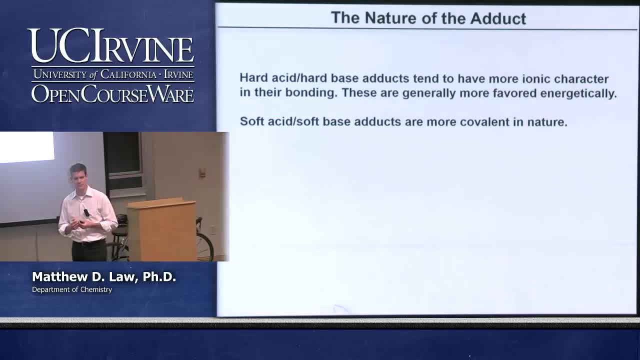 And you can imagine. this is more covalent nature, Covalent character. Okay, So I come in, I want a little bit of your electron density. You give it to me, We share it. Okay, And that's the covalent interaction. 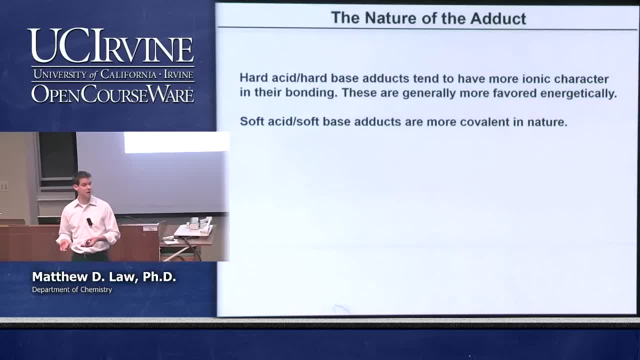 So soft-soft is strong, covalent, Hard-hard is strong, ionic, Good ionic, And the intermediates the hard-soft are not good at either one. Okay, And so that's why, in this kind of idea, very qualitatively, we expect the hard-soft to not be very favorable.